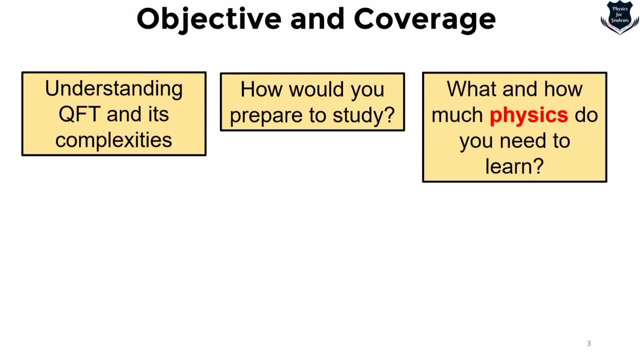 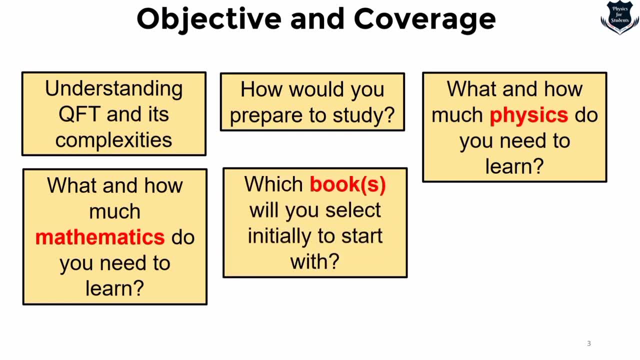 to study and, most importantly, what and how much physics do you need to learn? What and how much mathematics do you need to learn? What are the books that you will select initially to start with, and what are the mental preparations that you need to have? 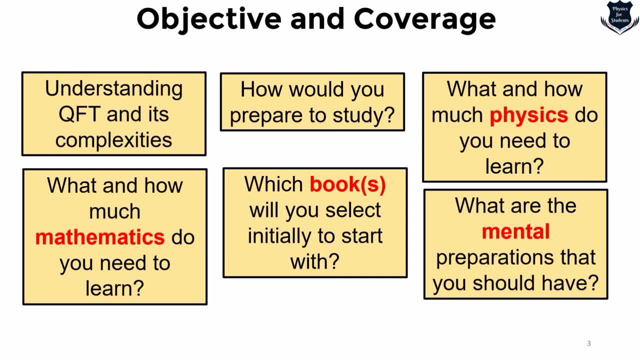 Now, overall, the video will comprise of dividing the entire concept of quantum field theory in this way. Now, why I have designed this plan is because this is the best way in which we can divide, understand, and then only we can understand the depths of quantum field theory and enjoy. 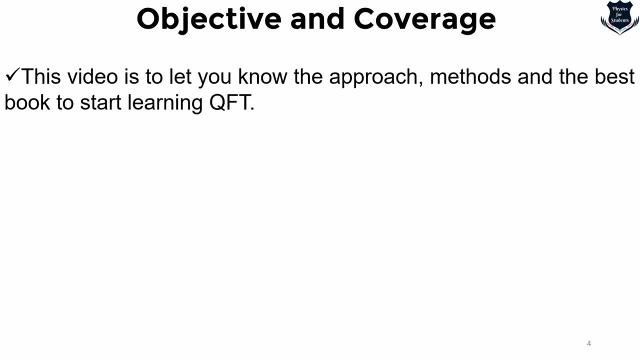 its beauty. So, first of all, this video will let you know the approach methods and the best books to start with, Books selection is a very big challenge because there are a lot of books on quantum field theory which are available. The target audience for this video can be 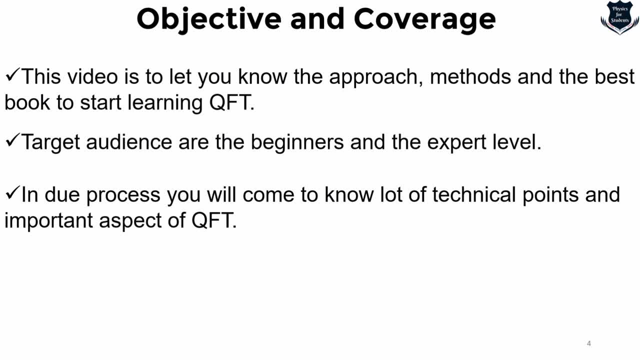 the beginners and the expert level. Now, in due process of time, although I won't be going deep into the mathematics chapter by chapter- but, yes, you will come to know about a lot of technical points, a lot of jargons and what is the meaning of those things. 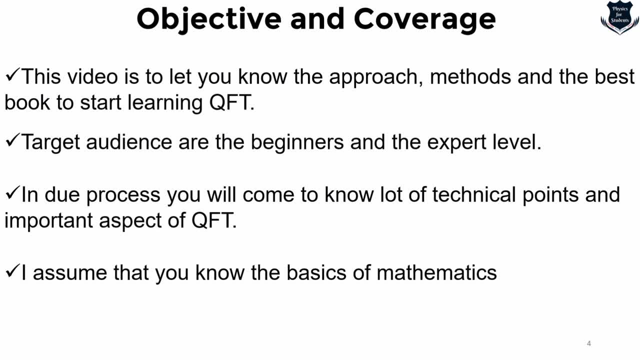 And, most importantly, I assume that you know the basics of mathematics, In general mathematics, which includes linear algebra, partial differential equations, little bit of set theory, basic mathematics, etc. So, having taken this assumption, now it is the time to explore the methods of learning quantum field theory. 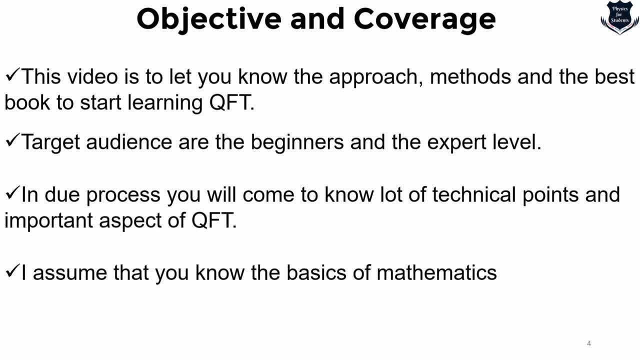 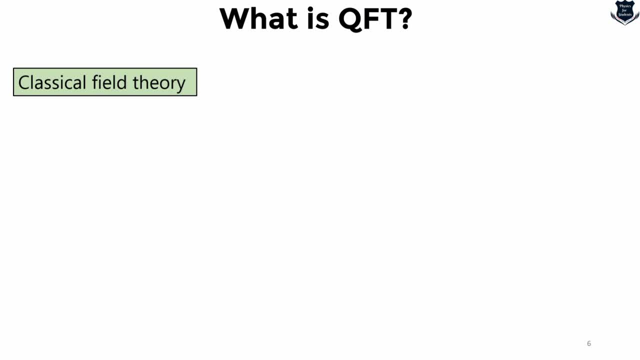 But before that, a very quick and a different kind of an approach to understand what is quantum field theory. Well, first of all, if we take as a whole, a kind of a pictorial description, quantum field theory is basically the classical field theory, along with special relativity plus quantum mechanics is what comprises of the quantum field theory. 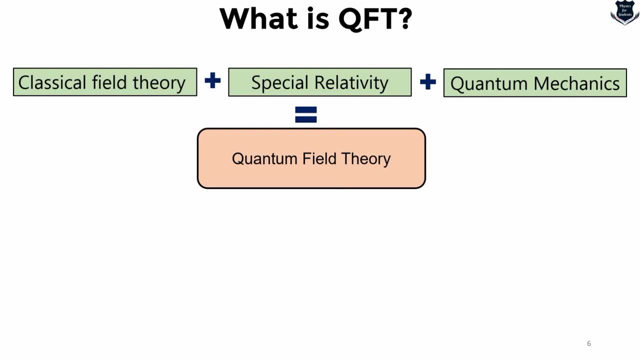 Now in theory, In theoretical physics. quantum field theory is a theoretical framework that combines classical field theory, special relativity and, obviously, quantum mechanics. Now quantum field theory is used in particle physics to contract physical models of subatomic particles. Now QFT treats particles as excited states. 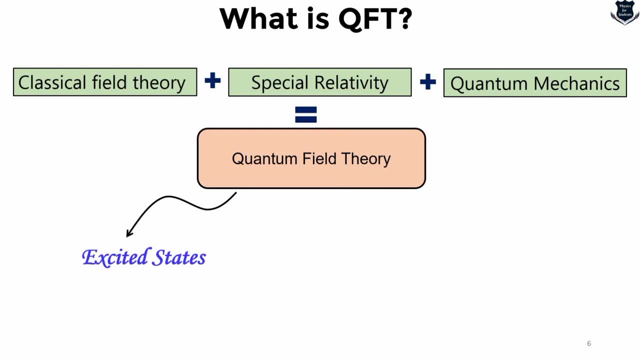 Yes, these are called quanta- of their underlying quantum fields, which is much more fundamental than the particles. The equation of motion of the particles is determined By the minimization- yeah, it is in the high energy- of the ground state. the equation of motion of the particle is determined by the minimization of the Lagrangian of functional associated by the particle interactions between, I would say, particles are described by interaction terms in the Lagrangian involving their corresponding quantum fields, and each interaction can be visually represented by what is called fine mind diagrams according to the perturbation theory of quantum mechanics. 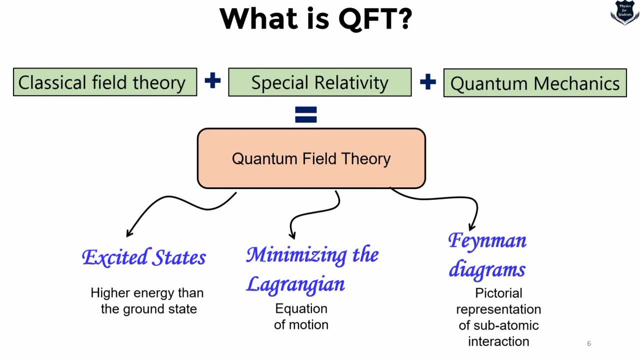 So in theory. So this is just a quick understanding of what is quantum field theory. it deals with excited states, it minimizes the equation of motion by using Lagrangian, and those are much more easily described by Feynman diagrams, which we will see in this video. 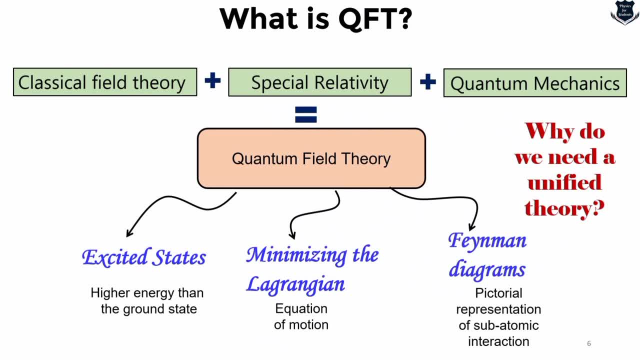 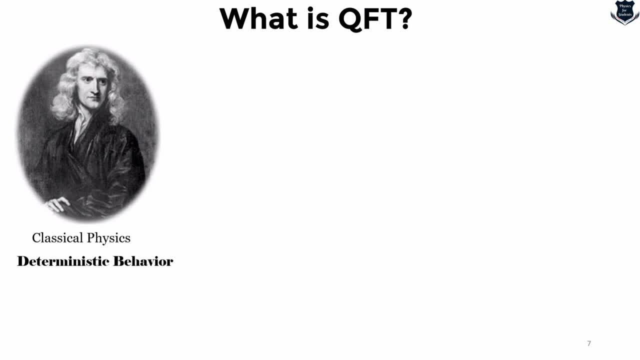 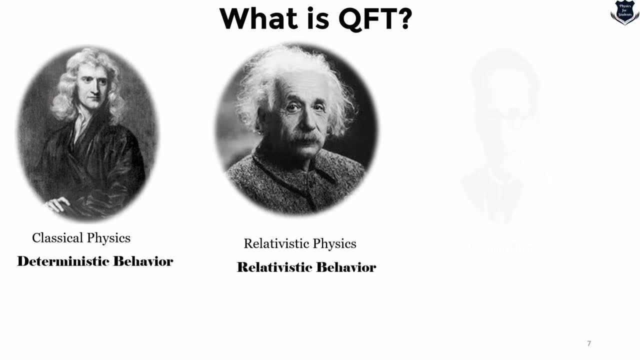 The question is that, again, because it unifies. the question is that: why do we need a unified theory, field theory? So, as we see that classical physics, which is guided by the Uh. deterministic behavior, along with the relativistic physics, which is guided by this relativistic behavior, and quantum physics, which is guided by the uncertainty or the quantum behavior, all these three things are actually merged into one unified theory. 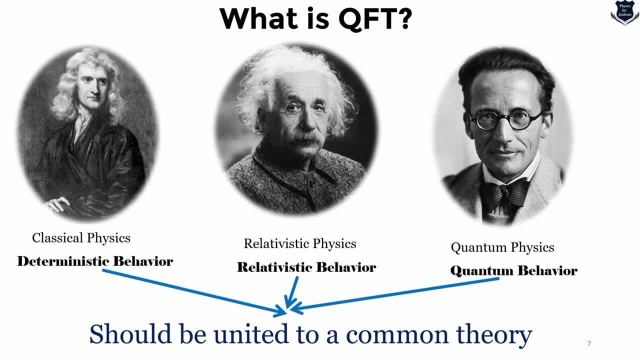 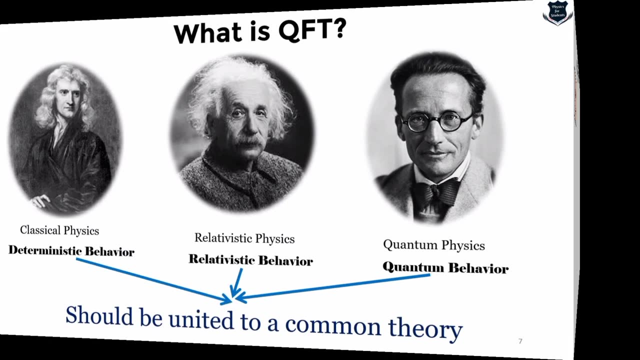 This is basically the target of unification. This is the area which we are all striving in order to get a unified theory, so that classical physics, relativity and quantum physics- the very big with the very small- is being united, and that is one of the objective of unification, and quantum field theory falls within those that unification. 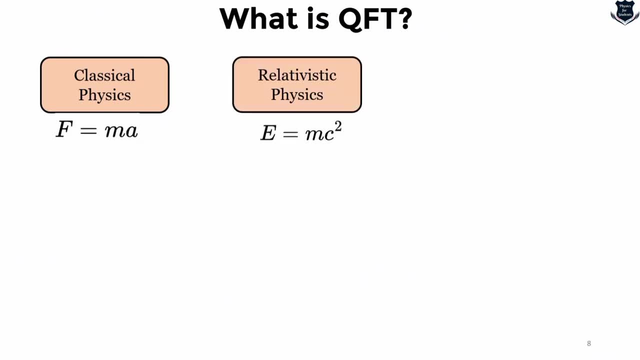 So you see, classical physics is guided by the famous Newton's formula, then relativistic physics by the equal to mc squared and quantum physics by the Schrodinger equation. and the very big, that is, general theory of relativity is guided by Einstein's field equation. 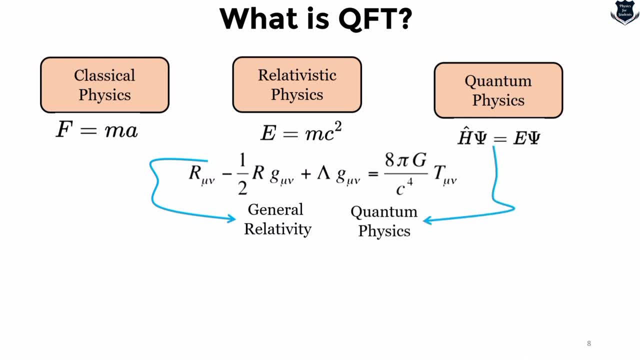 So, as you see, this is the general relativity and this is the quantum physics, and together, actually it comprises of this string theory that is a different part of unification, but it is quite okay to make a note of that that. this is actually general relativity plus quantum physics, comprises of the thing theory. 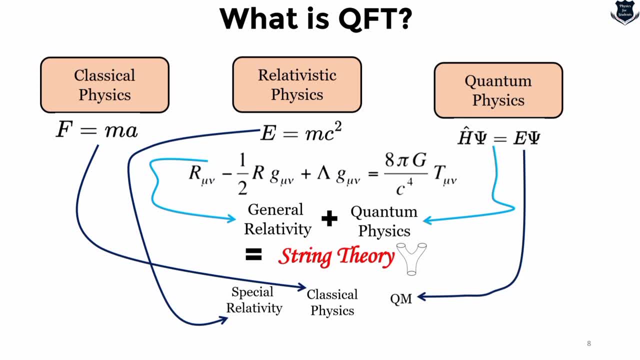 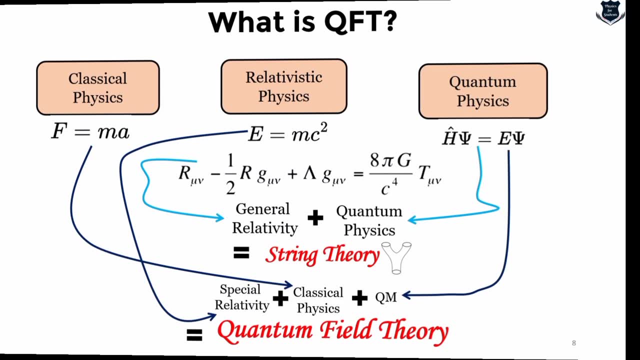 So classical physics, relativity physics- I mean it is a special relativity- and quantum mechanics together mix up what is called the quantum field theory. Now, I have already made a video on this so you can have a watch. 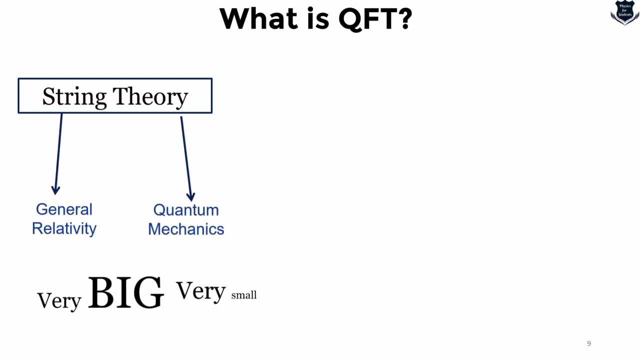 So here it is. string theory is general relativity plus quantum mechanics, uniting the very big With the very small. quantum field theory comprises of special relativity, classical field theory and quantum mechanics. Again, quantum field theory can be divided into parts, that is, quantum electrodynamics and quantum chromodynamics. 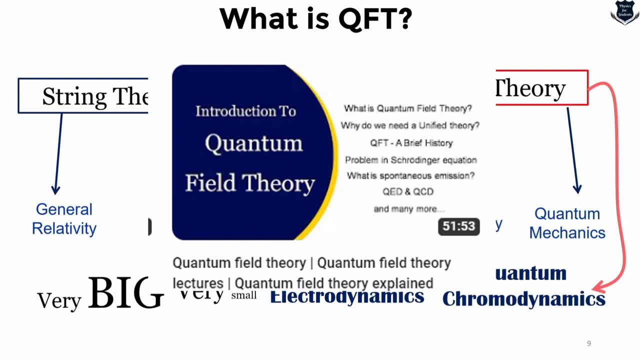 This is the video which I was talking about. You can have a look into this. This is a much more detailed video, only speaking on what is quantum field theory, a little bit about the history. why do we need unification, Schrodinger's equation and a lot of details into what is quantum electrodynamics and chromodynamics. 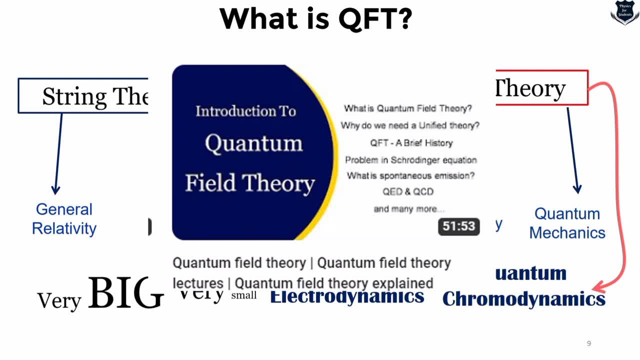 You can go there in my channel, Physics for Students. It is a detailed video, so it comprises of the entire details of quantum field theory. We understood what is quantum field theory in a nutshell. Now the question is that whenever we need a new theory, there should be a limitation for the earlier theory. 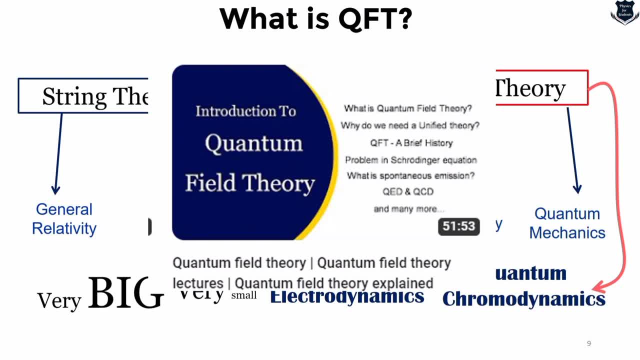 There should be some areas which we cannot understand or we cannot depict in mathematical or intuitive ideas. What is the limitation of quantum mechanics which led to the foundation of quantum field? We will look at quantum field theory coming up into the next part of our video. 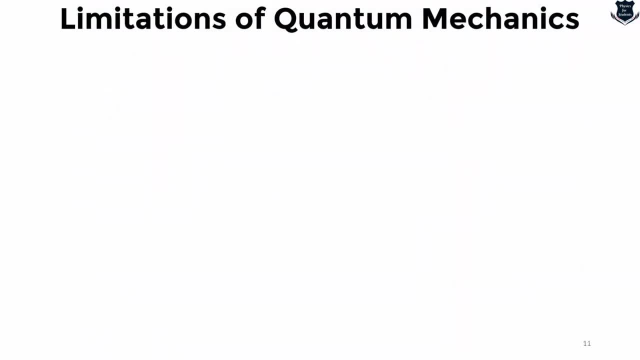 So we will look a little bit quickly into what are the limitations, what are the problems with the quantum mechanics. Now, you see, quantum mechanics initially started and it treats as a single particles That means, say, for example, an electron, basically in a potential, for example square, well, harmonic, oscillator etc. and actually it retains its integrity. 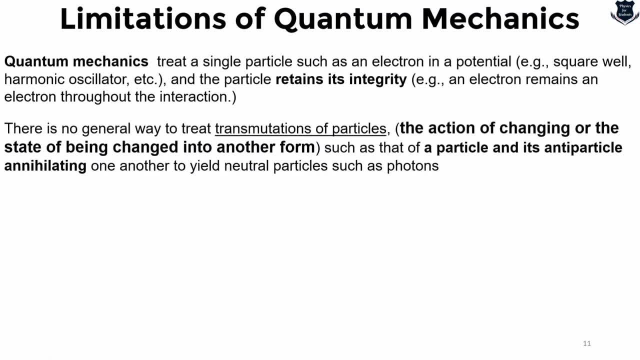 And there is no general way in quantum field theory which is called to demonstrate. So, for example, in quantum field theory we can define a transmutation. What do I mean by transmutation? It is basically the action of changing or the state of being changed into another form. 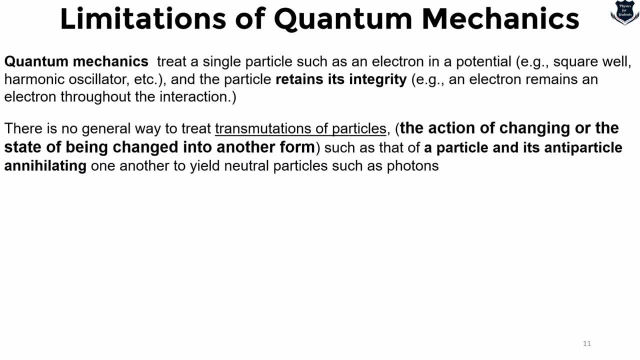 One particle being changed into another form, such that of a particle and its antiparticle annihilating into one other, can be described. So you can think this is a kind of a limitation right. So for example, this one, it is a kind of a change which was not defined. 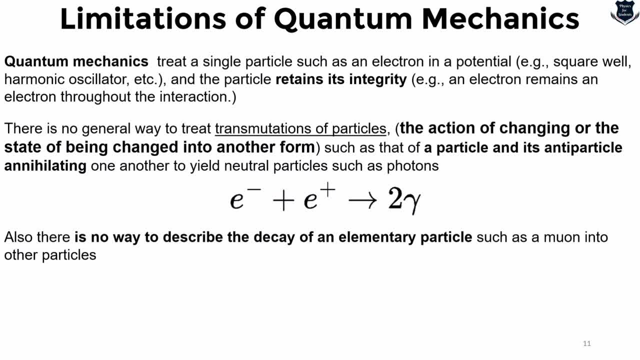 So anyway, the electron and the positron say, for example, giving rise to another particle, And there is also no way to describe an elementary particles decay, such as muon, which is getting decayed into another particles. These were not being properly defined into quantum mechanics. 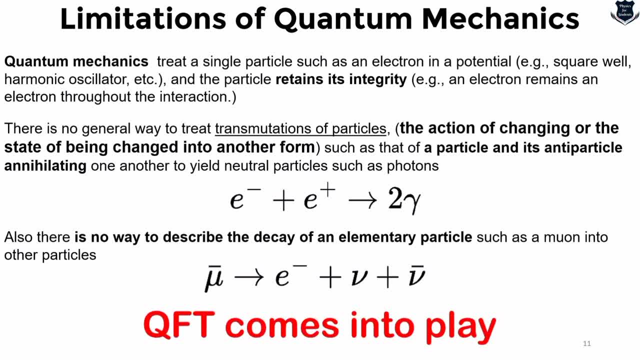 For example this one. So this is where quantum field theory actually comes into play. That means defining not only the subatomic particles as what I would say as particles, or retaining as potential, But one particle, One particle transmuting into another, and defining what is called the particle decay. 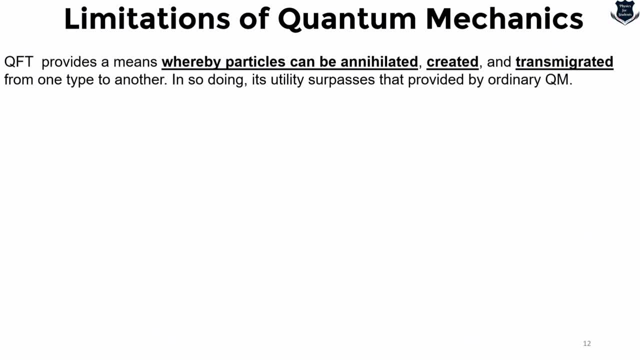 So here comes quantum field theory. So you understand that it provides means whereby particles can be annihilated, created and transmuted or transmigrated from one type to another. So if I consider, for example, this kind of a interaction where an electron and positron, that produces a muon and an antimuon, 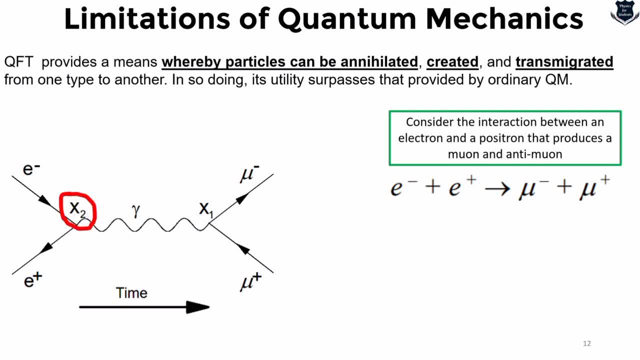 Definitely we can define that using a Feynman diagram. So at this position x2, I can say, the electron and the positron annihilate each other to produce a photon, And in this position x1, the photon is transmuted into muon and an antimuon. 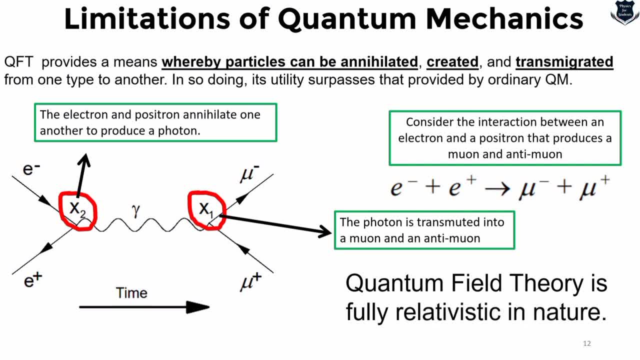 So this is basically what is, and another important is that quantum mechanics was not relativistic. Quantum field theory is fully relativistic, Right, So we can think of this interaction as an annihilation of the electron and the positron at the position x2.. 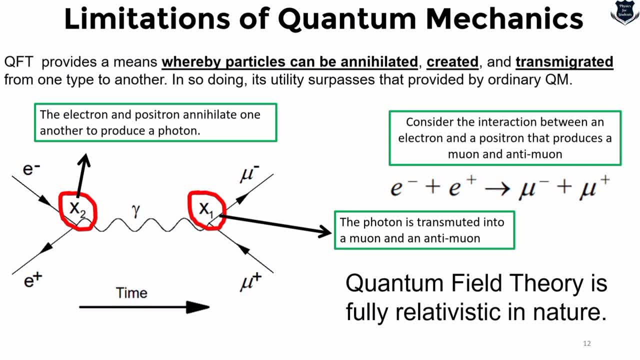 Accompanied with the creation of photons and that followed by the destruction of the photon, accompanied by creation of muon and an antimuon at position x1.. So, unlike the incoming and outgoing particle, in this example the photons as you see here, denoted by gamma sign, is not a real particle. 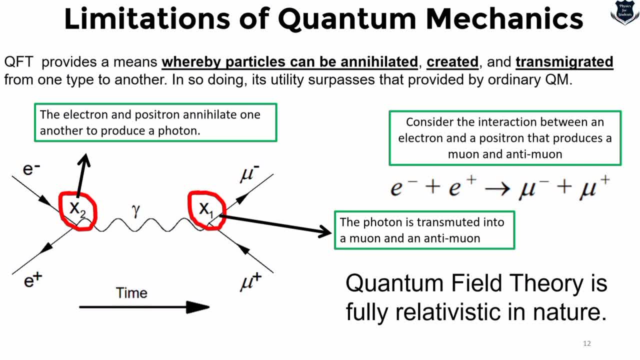 But it is actually a transitory or you can call it as a virtual particle. So this is actually what is the limitation and why quantum field theory came into being, And this is extremely important Before we go and jump into understanding the complexities, books or sources that what was the limitation of quantum mechanics and what gave rise to the birth of quantum field theory. 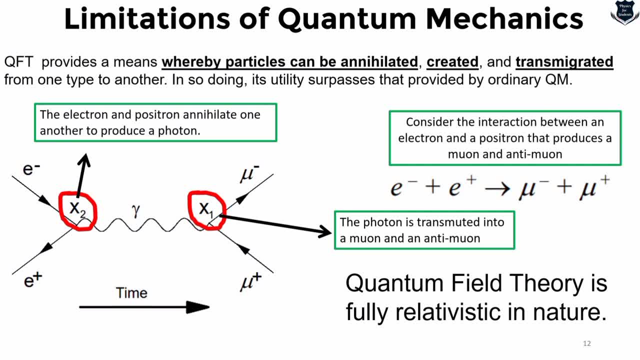 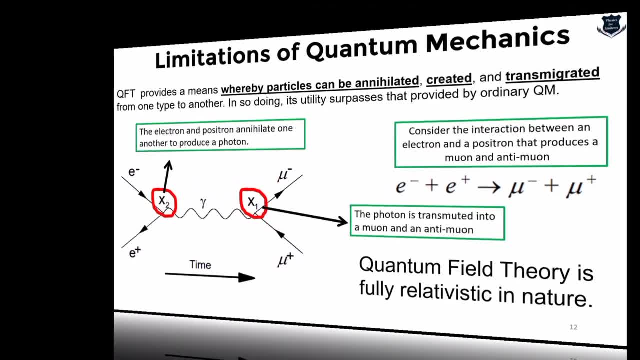 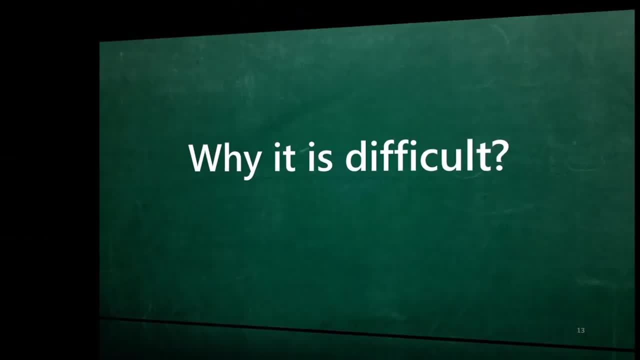 Now, apart from all these things, we should have understood the basic thing which keeps the students and all of us constantly perplexed. is that why it is difficult? Let us find out into this part of the video. Understanding difficulty is important. Based on that, we design the strategies. 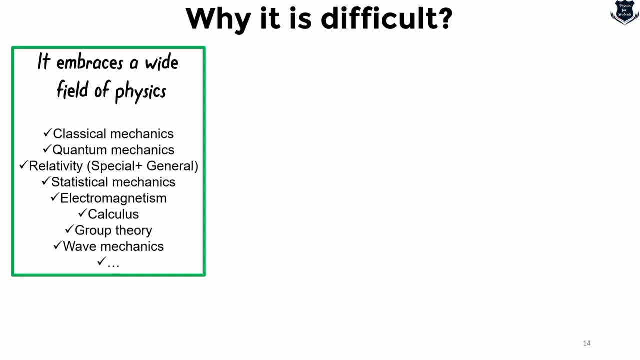 So the first thing in this: You see, quantum field theory actually embraces a huge field of physics, So you need to have an understanding of classical mechanics, quantum mechanics, relativity, including a little bit of general, Then statistical mechanics, electromagnetism, lot of mathematics, etc. 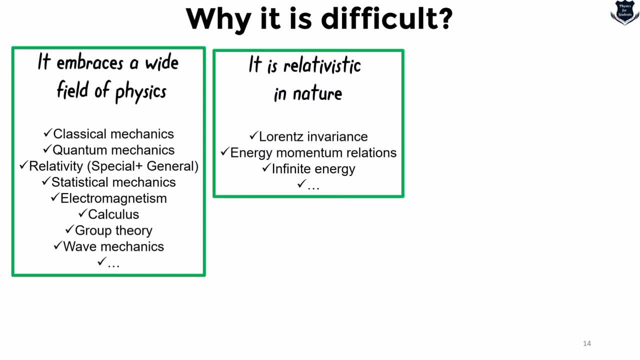 The second part is that it is relativistic in nature. That means each and every equation of quantum field theory has to follow the Lorentz invariance, has to follow the energy momentum relation, has to follow what is called infinite energy momentum. 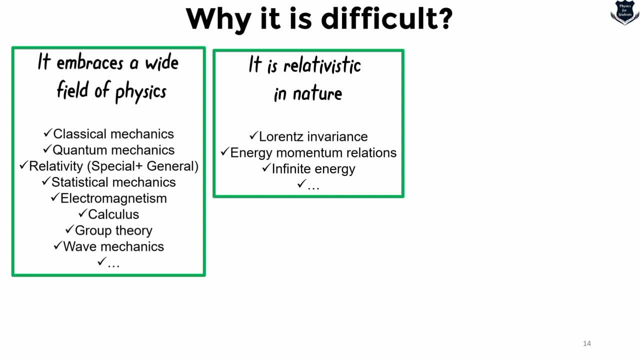 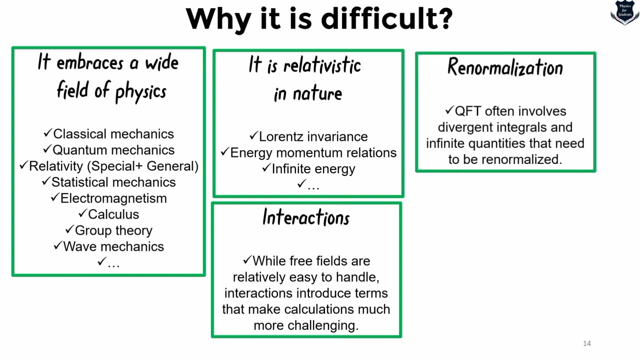 Has to follow what is called infinite energy and lot of other postulates and rules. The third thing is that interactions- Free fields are relatively easy to handle- Interaction- introduce terms that make calculations much more challenging, Because if you are dealing with infinity, if you are dealing with interactions among lot of particles in a wide spectrum of space and time, obviously there would be some problems. Yes, This is one of the biggest challenge of quantum field theory: Renormalization. That means there will be infinities, there will be problems and we need to renormalize so that the infinities are cancelled out and we get something very comprehensive. 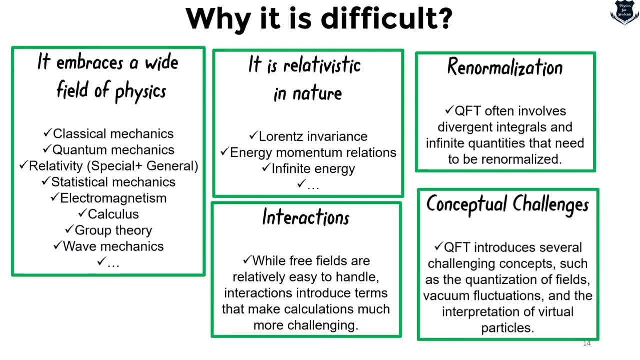 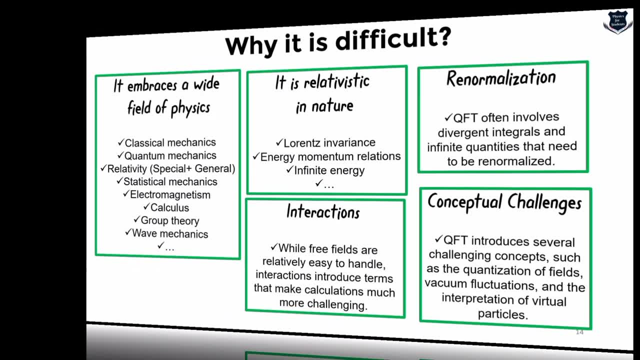 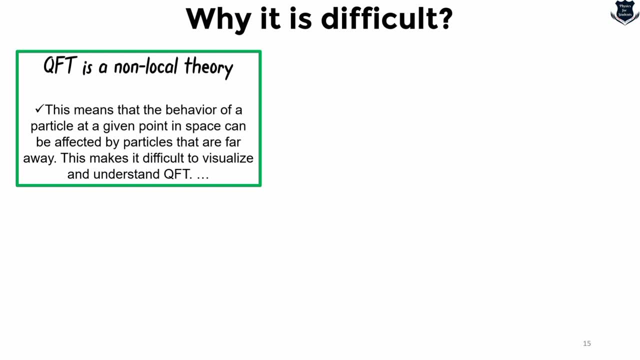 Obviously, the conceptual challenges are there. Quantum field theory introduces challenging concepts like quantization of field vacuum, fluctuations and lot of other things. The other difficulties include what is called it is a non-local theory. That means we know that you know what is a local and a non-local. 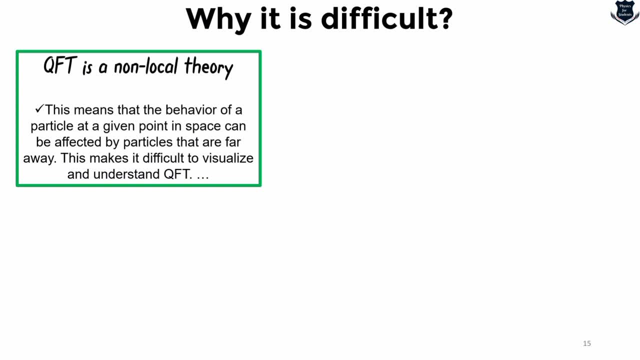 I don't think I need to explain, But yes, It actually is about the behavior of particles at a given point in space, which can be affected by particles that are far away. So it is not that one particle is leading to another equation, and so on, and so on. 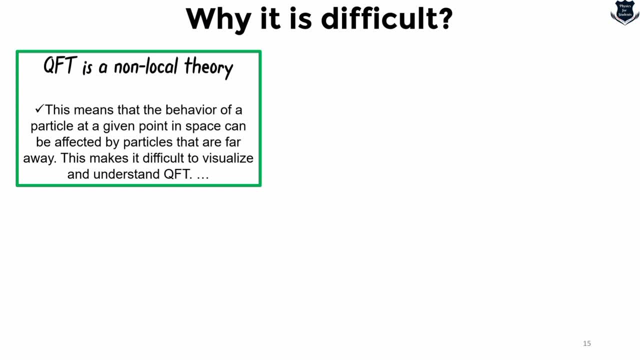 So this particle, because it is a field theory, it is a wide area of space and time, will be affected by other areas. So we have to visualize, we have to design a mathematical tool because of this non-locality. Well, experimental verification. 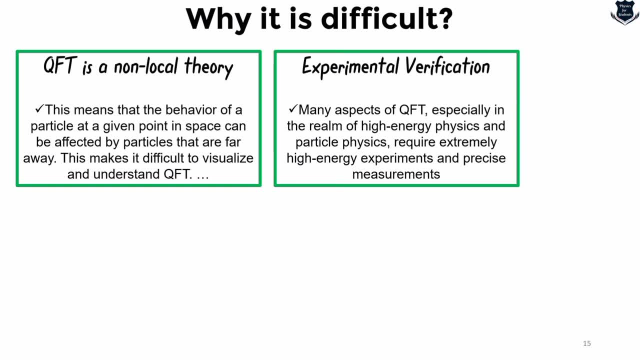 Many aspects of QFT. When we are dealing with high energy, physics has not been experimented. The particle accelerator, etc. does not always produce the exact amount of energy which is required, So that makes things different. So this is the last one. 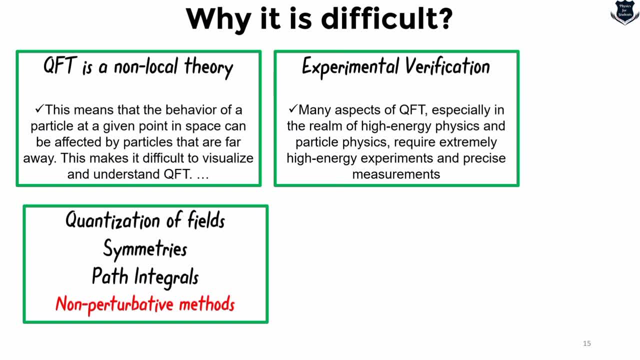 Quantization, symmetries, path integrals and non-perturbrative methods. Now, why I have made it red is because I am going to explain what is a non-perturbrative method, Because this is, again, very important in your understanding of how to learn quantum field theory. 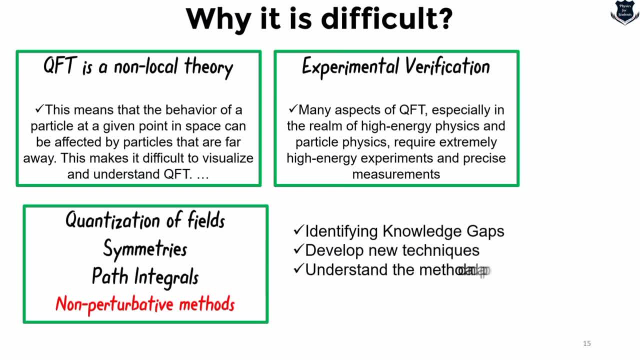 So you see that you might be wondering Why I am telling You need to identify the knowledge gaps. That is why we can develop new techniques, understand the method and approach and design it accordingly. So you will see, most of the time we again and again have to revisit the classical field theory, classical mechanics, maybe quantum mechanics, again and again. 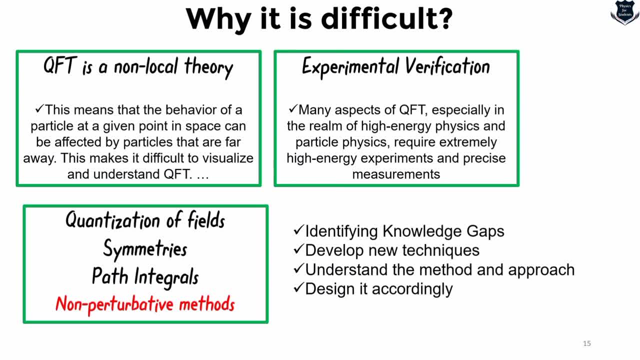 Because, based on that, the extrapolation has been done and modified into a generalized theory called quantum field theory. So we have to identify and bridge the knowledge gap and develop the new techniques. So that is why this is extremely important. What is important is that this question 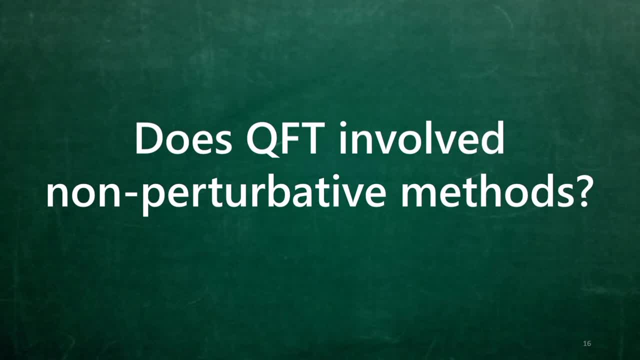 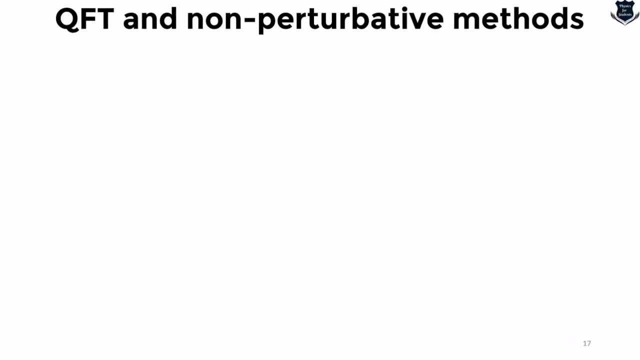 Is. quantum field theory involves non-perturbrative methods Coming up into this part of the video. Before going into this, I would like to quickly explain you what is a perturbation and what is a non-perturbration. Now, if I take quantum mechanics as a whole, 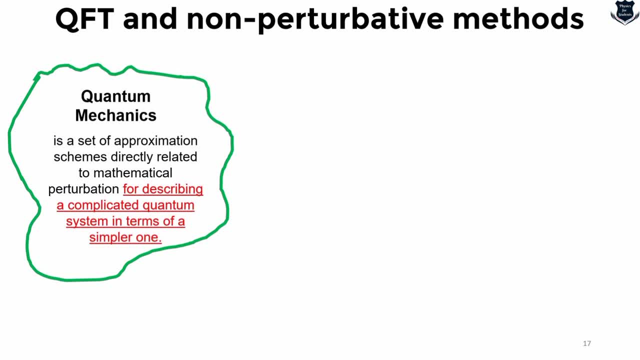 As a whole, then you will see that there sometimes comes a very complex quantum system. Always, exact solutions are not possible, Exact values are not possible. So what we do is that we set a kind of an approximation scheme, And this is what is called a perturbative method. 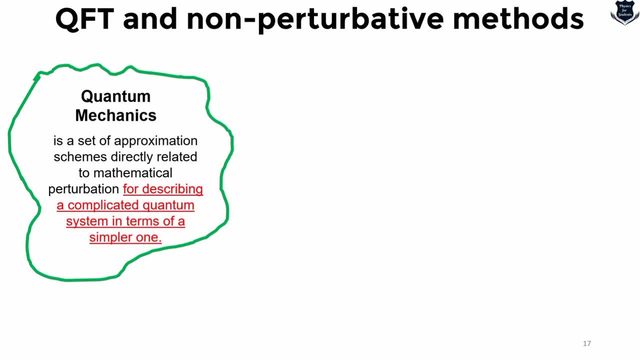 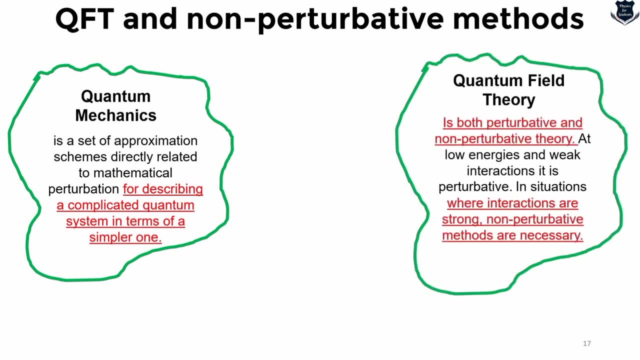 Perturbation means disturbance. Things are moving, So we cannot get a complete understanding. So we define what is called a perturbative method. Now you see, the problem is that quantum field theory is both perturbative. That means a kind of an approximation is given. 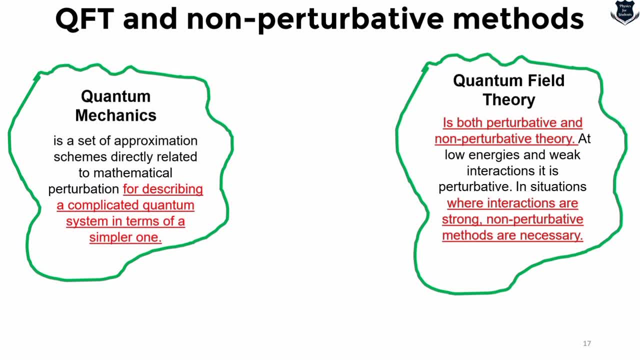 As well as non-perturbrative. That means we require an exact value of the complex quantum system. So at low energies and weak interactions it is perturbative, obviously, But in case of where interaction is strong, Where it is high energy. 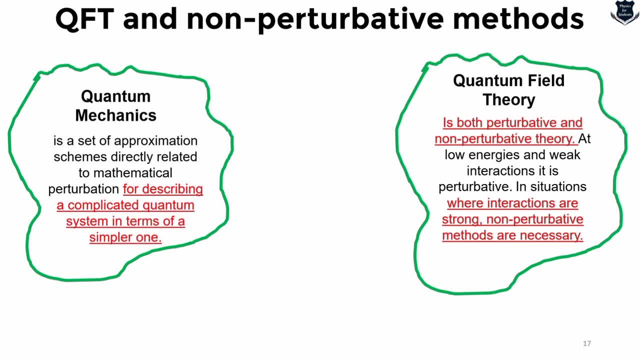 It is, non-perturbrative Methods are necessary. Now, that is what we need: to go beyond the perturbation theory. Perturbation is, you know, easy, We get an approximation. But we have to go beyond the perturbation theory And we have to make it certain. 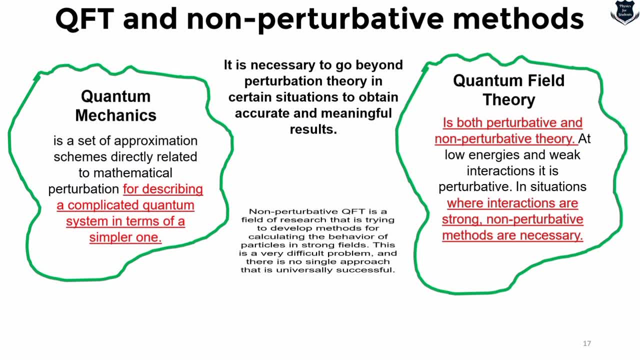 That we get an accurate and meaningful results. So non-perturbrative theory, of Non-perturbrative quantum field theory is actually not yet designed, But there are researchers, There are problems, There are solutions which are going on. 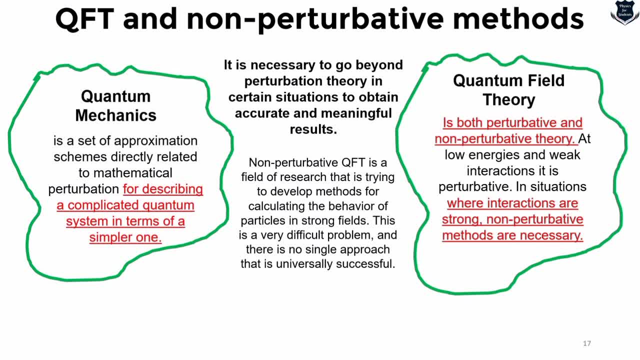 And this is a very single, unique problem, Because getting such a wide expanse of field And getting you know kind of a non-perturbrative method, That is, finding a single value- It is very difficult. So these are the theories which are going on. 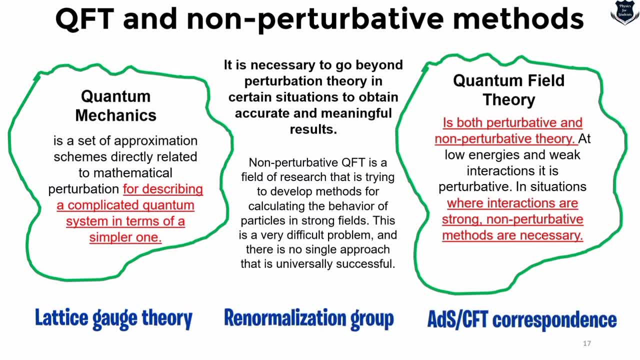 Lattice gauge theory, Renormalization group And the ADS-CMT model. Now, that is why, again, you understand the complexities of quantum field theory Is not only due to this, But also due to finding out a non-perturbrative solution. 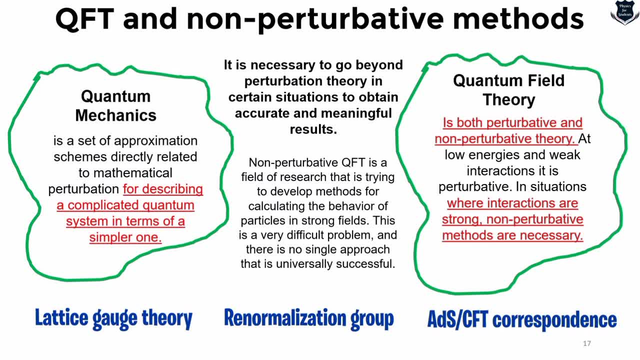 The question is that Why do we need a non-perturbrative method? I mean to say There should be a proper reason. Let us find it out In the next part In this section, Where we are going to look into. 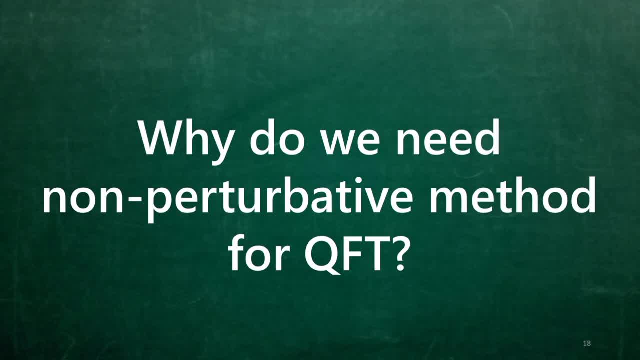 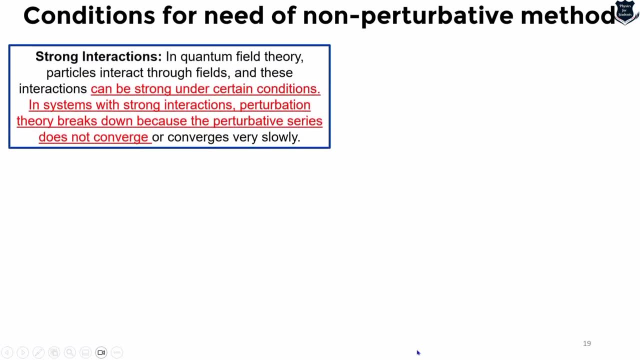 Why at all quantum field theory Needs a non-perturbrative method, Coming up into the next part of the video. So So you see that the first thing is that The strong interactions Which sometimes come in quantum field theory, 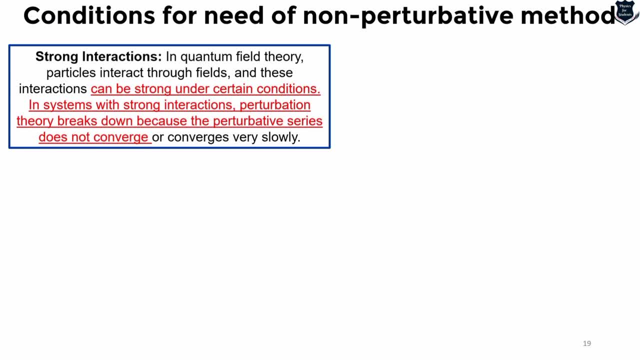 Here. What happens is that the perturbation theory breaks down And the perturbative series Always do not converge. So for that we need what is called Non-perturbrative theory. The second thing is that Quantum chromodynamics 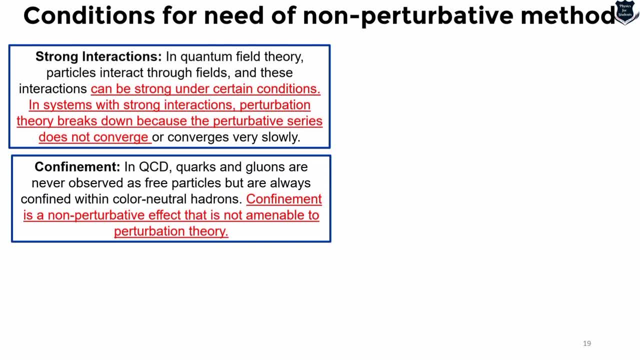 Which is again a One part of the quantum field theory. The confinement are actually non-perturbrative effect. So that is not amenable to perturbative theory, Because free particles are always Confined with color neutral hadrons. 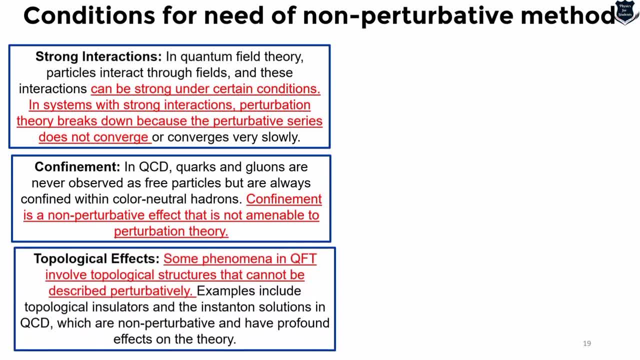 I am not going into these details, But this is something which is required. Also, the topological effects. Now, some phenomena, Some occurring in quantum field theory, Involve topological structures Which definitely cannot be described by Perturbrative method. 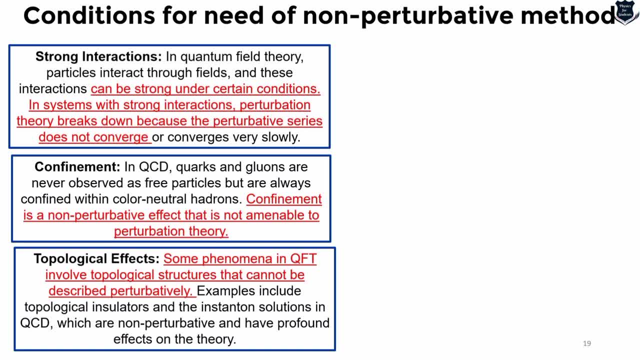 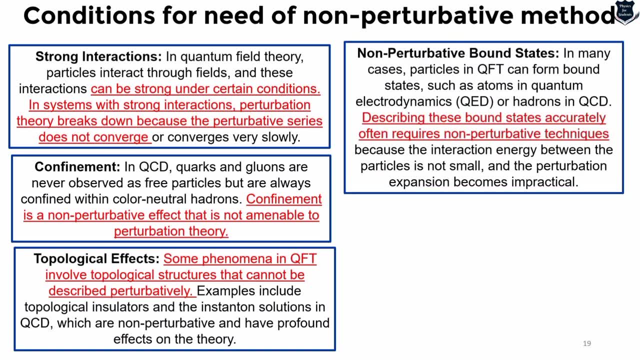 So, which includes, like topological insulators And instant and solutions in quantum chromodynamics, Which needs a non-perturbrative theory And a profound effect on the theory. Also, in many cases Particles in quantum field theory Can form bound states. 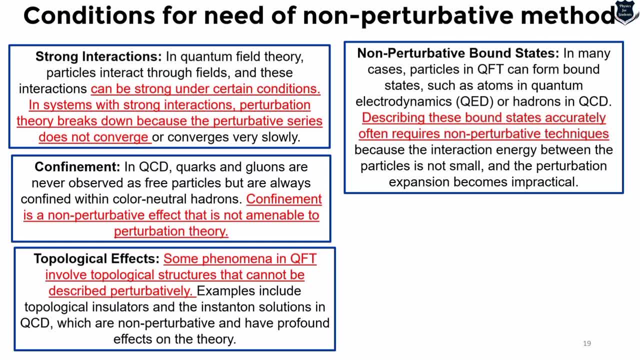 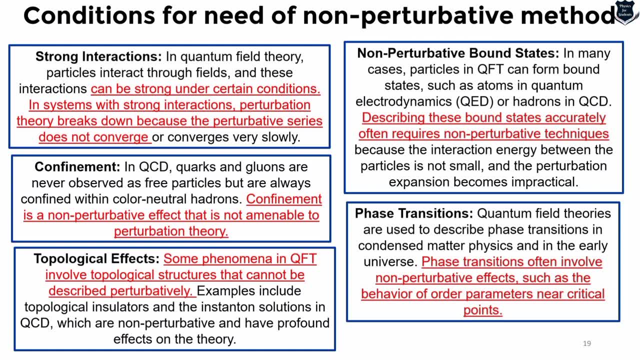 So, in order to describe These type of bound states, We need what is called A non-perturbrative technique And, obviously, the phase transition, That is, quantum field theories Used to describe different phase transitions In universe. So phase transitions: 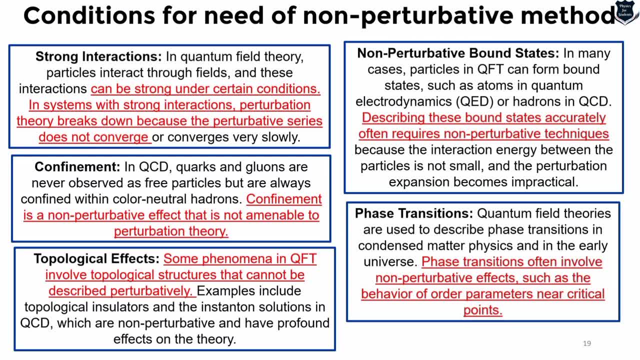 Always involve, I would say, Non-perturbrative effects And the behaviour of order of parameters Near critical points, And there are several other examples. So 1, 2, 3, 4, 5.. These are the 5 quick examples. 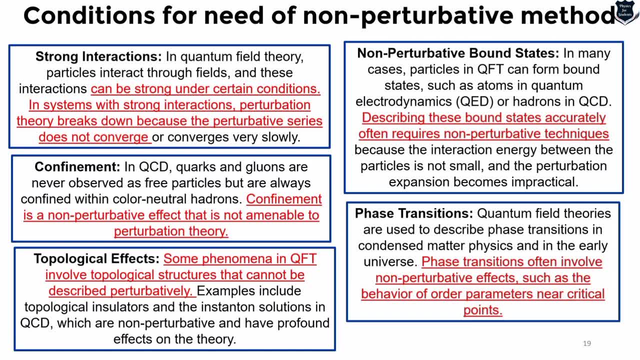 That why quantum field theory Is not depending on the perturbrative method, But needs to have something very accurate, Something very clear, And we need to identify Through non-perturbrative method, Which becomes extremely difficult and complex. 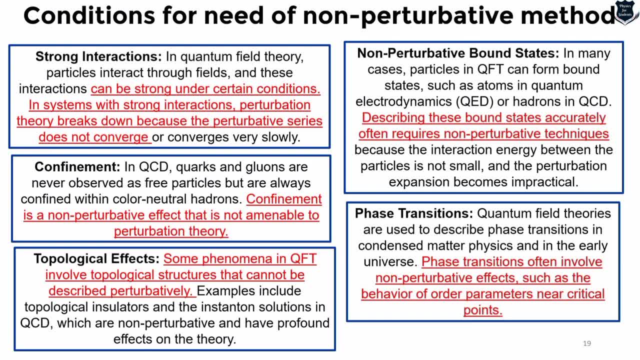 Because the wide area It is filled not into particles. Now it is a time That we should start preparing For quantum field theory: How to understand, What are the loopholes that we have, What are the books And what are the things that we should look into it. 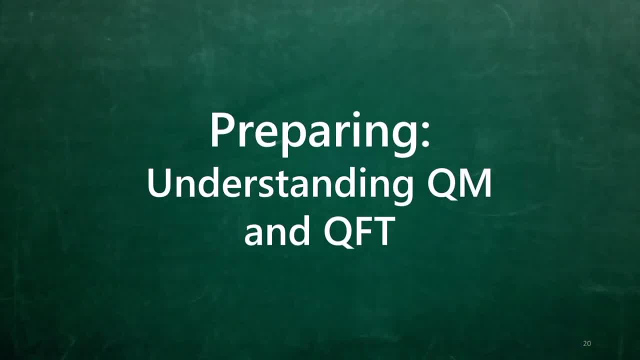 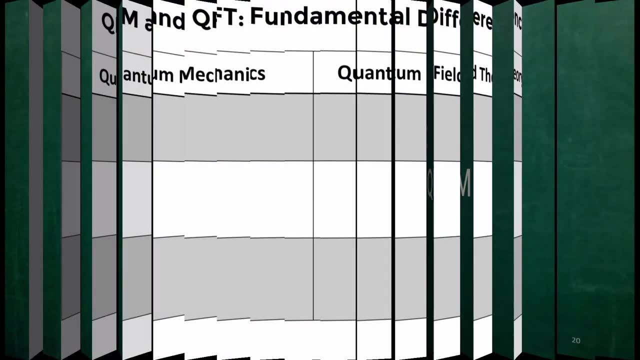 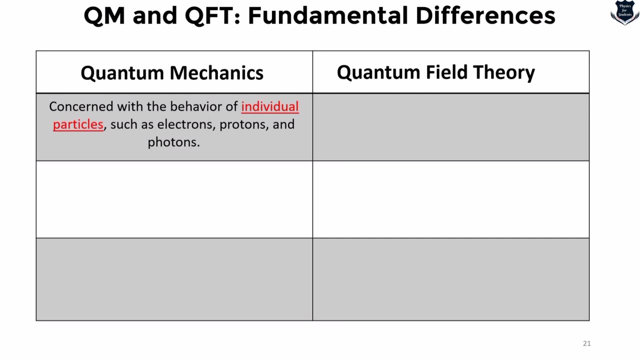 Coming up into the next part of our video, Preparing quantum field theory, And before that We need to understand That what quantum field theory offers Which quantum mechanics do not offer. This is central. This is important in understanding So that the gap is eliminated. 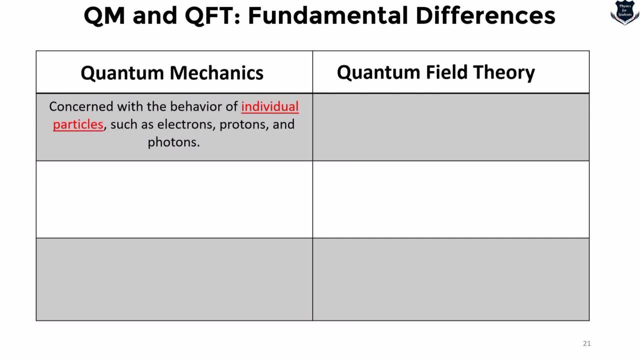 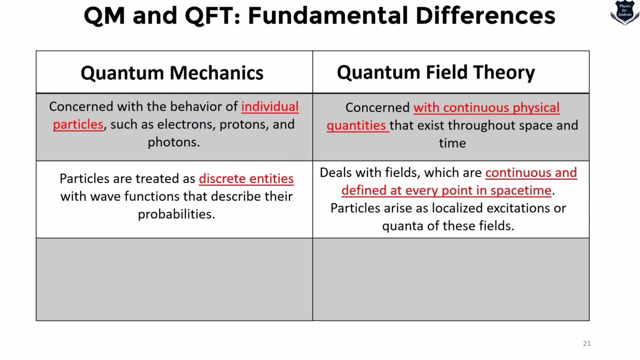 Quantum mechanics deals with Individual particles- Protons, electrons, photons, etc. And quantum field theory is spread out. It is continuous physical quantities That exacts through space and time. The particles are also called Discrete entities And that is why you use the greek letter psi. 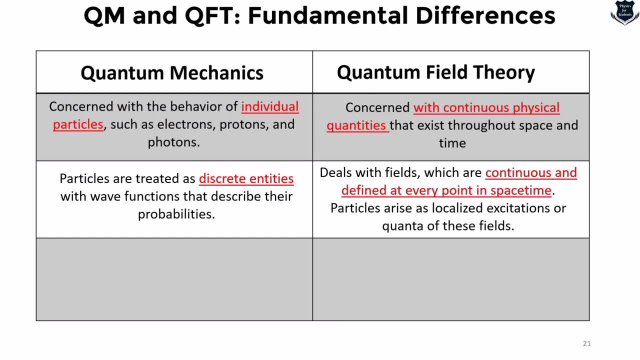 So that we can denote the wave functions. But it is not here. QFT deals with continuous space time. That is defined in every point And particles arise as Localized excitations. I just mentioned it right at the beginning of the video. 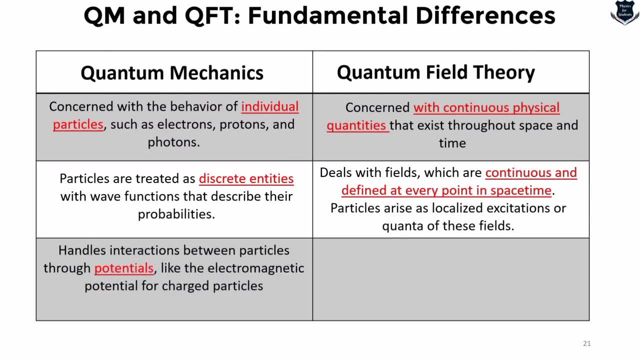 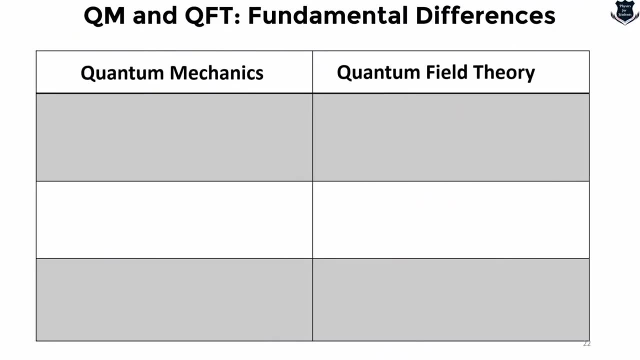 It handles interaction Between particles through potentials, Mostly electromagnetic potentials And other things. Here in quantum field theory It incorporates between fields, So these interactions are described through terms, In terms of field equations. Next, what we see That in quantum mechanics 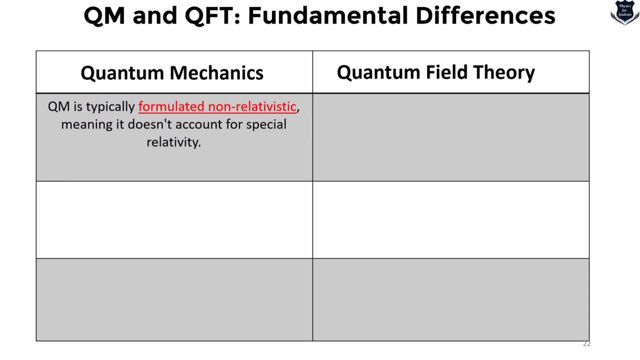 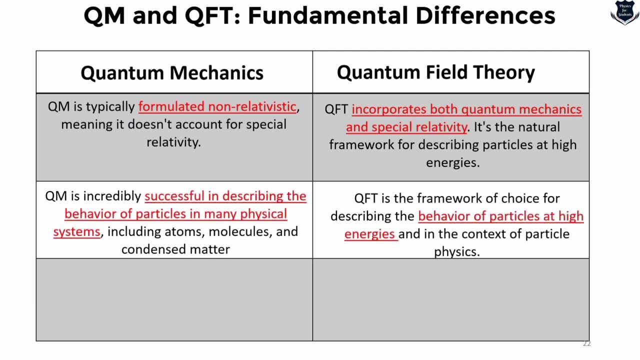 What we find is that It is obviously not relativistic in nature. That is one of the basic reasons That we formulated quantum field theory, Because it is relativistic in nature And quantum mechanics Is incredibly successful In describing behavior of particles. 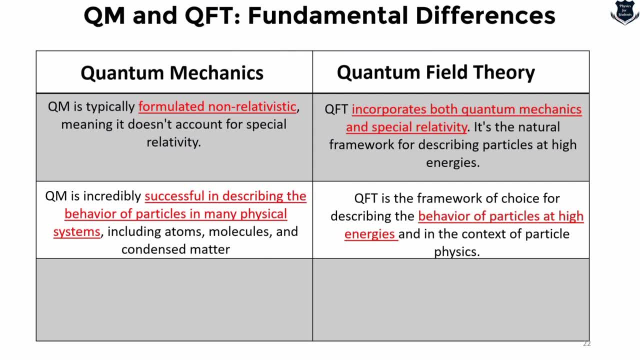 In many physical systems. But here quantum field theory Is a framework which describes That high energy physics, Because it incorporates special relativity And lastly quantum mechanics, Actually treats point like objects, Where quantum field theory Deals with excitations of fields. 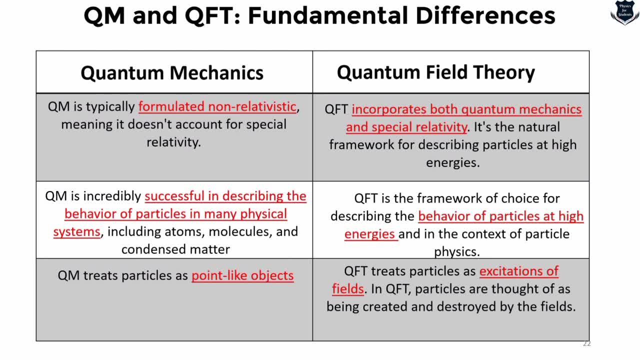 And quantum field theory Is annihilated by the fields. Now, you see, that is why, Once we understand the difference, Then when we are reading quantum field theory, When we are visualizing and encountering Those big equations, We won't face a problem. 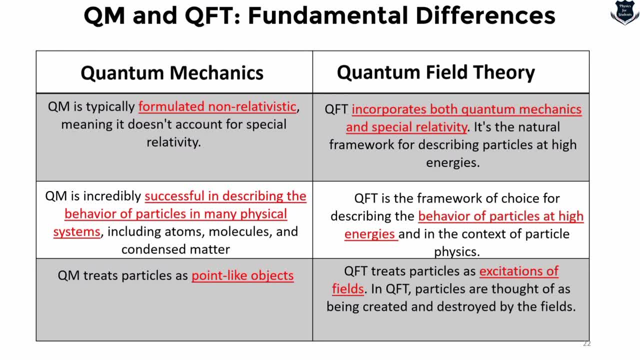 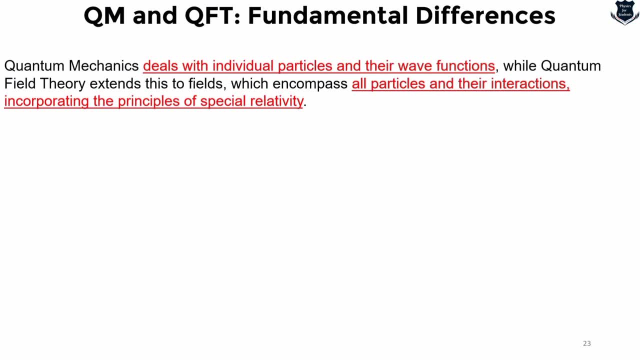 And that is why I stated the difference Between QM and QFT, So that these things become clear. Also, you will see that quantum mechanics Deals with individual particles and wave function, While quantum field theory Is basically interaction of particles In between them. 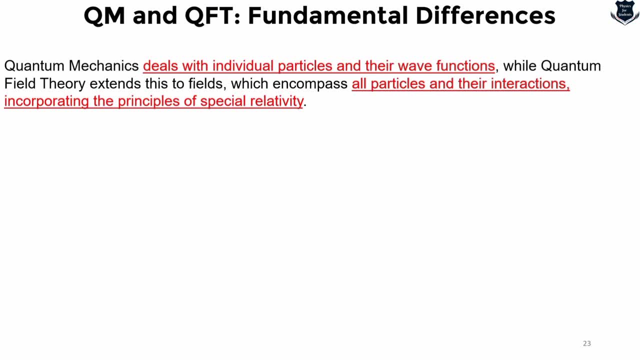 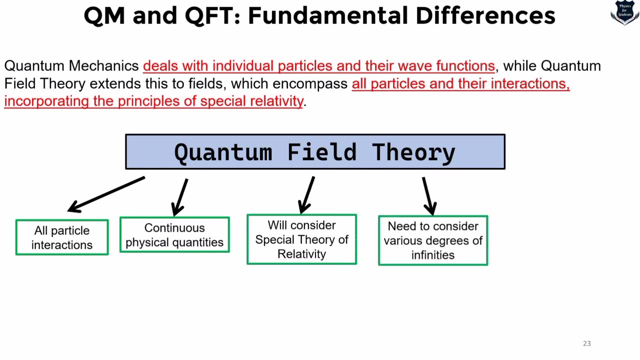 And it incorporates The special theory of relativity. Now let me show you A bigger holistic picture. So if I take quantum field theory, You see it incorporates number one: All particle interaction. It incorporates continuous physical quantities. It also takes special theory of relativity. 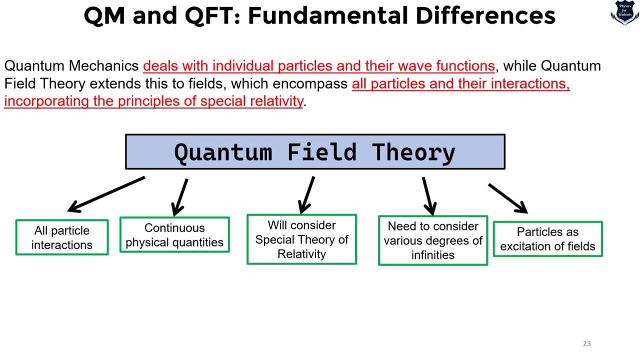 And you need to consider Various degrees of infinities, And the particles are considered more As an excitation of fields. So now, once you get a holistic picture, It helps us to understand Quantum field theory And thereby understand And prepare accordingly. 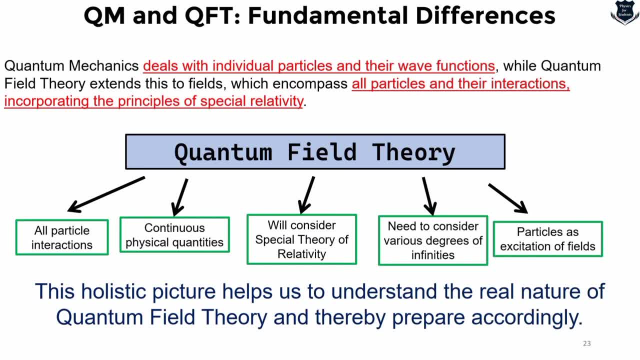 So this part of the video, We understood the knowledge gap, The difference. What is quantum field theory, Why it is requiring a non-motivative methods, And so on. Question is that: how will you prepare? What are the areas that you should first study? 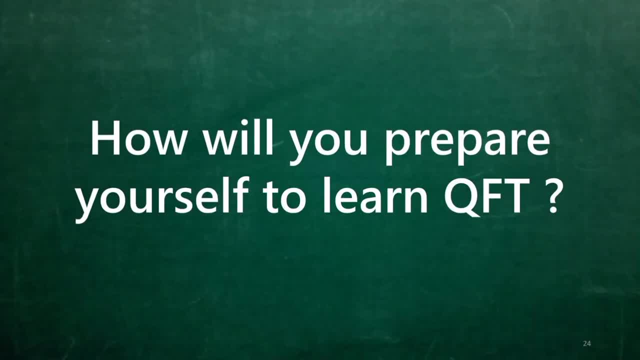 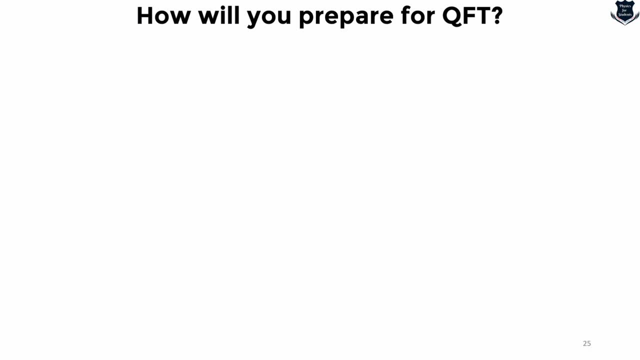 Second, etc. What is the way that you do? Coming up into the next part of our video, I will divide this part into small, I would say, blocks, And then go block by block So that we can overcome those difficulties. First is that we need to understand. 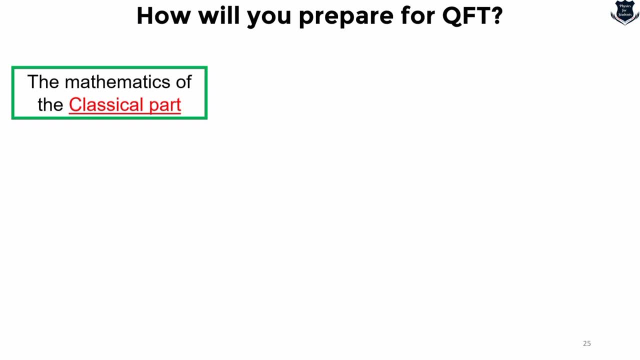 The mathematics of the classical part. Now you are wondering Why I have made it red and underlined, Because this is again most overlooked And students and we think that, okay, We are done with classical mechanics In our school days, So we can immediately jump into quantum field theory. 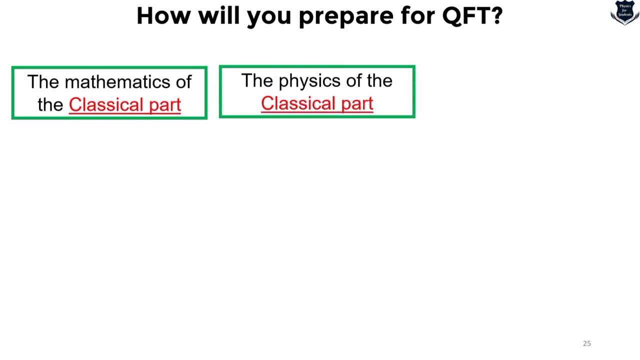 It is not. We need to understand the physics of the classical part. Not all of them, But some of them. What are those? I will just tell you now. We also need to get into the physics of the modern part And the mathematics of the modern part. 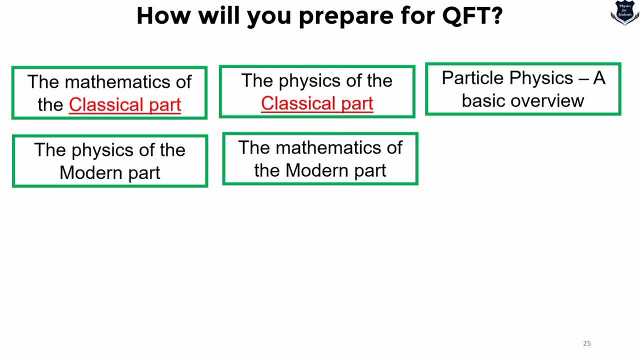 Apart from that, we need to have a good idea Of the basic idea of particle physics And overview And quantum field theory. If, single, we are selecting Which is the best book to select- And yes, the most important factor Is that selecting the right book- 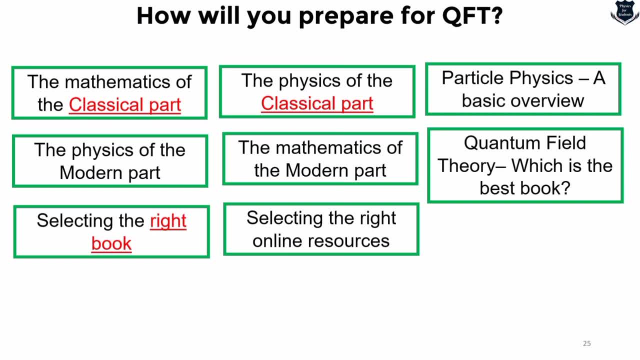 Now, if you have What are the right online resources, That we will do So. we will divide it into this 3 plus 3 plus 2. 8 blocks, And then we will go block by block, Understanding the videos, The books. 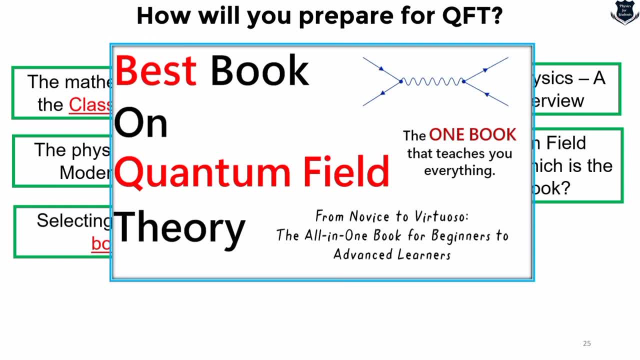 The preparation Now, if you have watched my earlier video Which I launched just last week, What is the best book on quantum field theory Where I have detailed? Have a detailed discussion On Eberhard Seidel's book on quantum field theory. 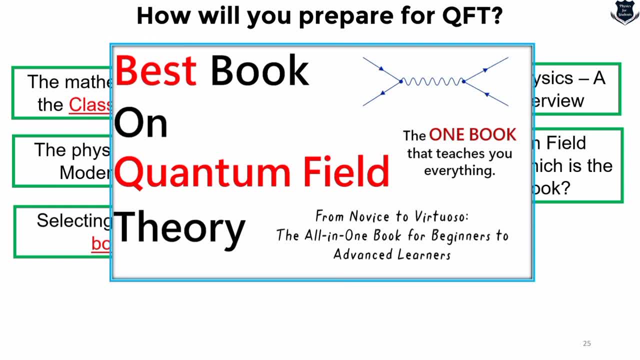 But this Is going much more into the blocks And giving you much more details. Now, apart from these things, You might be feeling a little bit pessimistic. That do I have to go through all those mathematics Again and again? No, 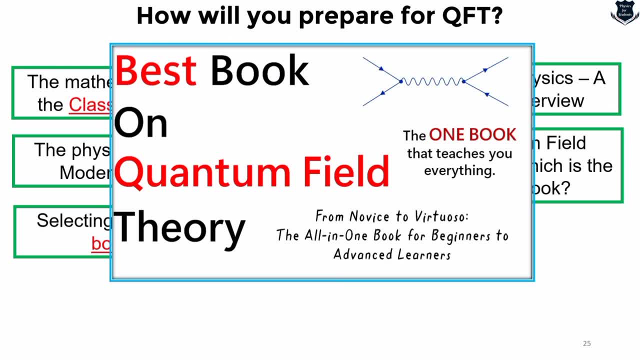 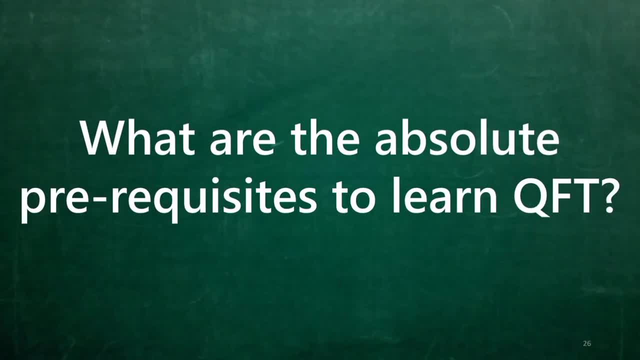 There is something which is called an absolute prerequisite For quantum field theory. I mean to say, you need to have that much only, And you can jump into that. What are the absolute prerequisites for quantum field theory? Coming up into the next part of our video, 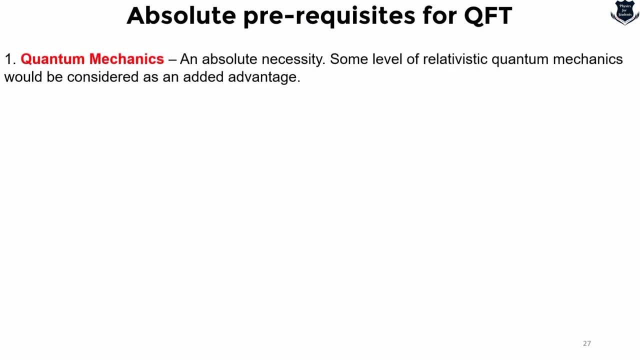 So first of all, You need to see that quantum mechanics- No doubt this is absolutely The first stepping stone, And you need to have a little bit idea Of relativistic quantum mechanics. It can be considered an advantage, But knowledge of quantum mechanics is an absolute necessity. 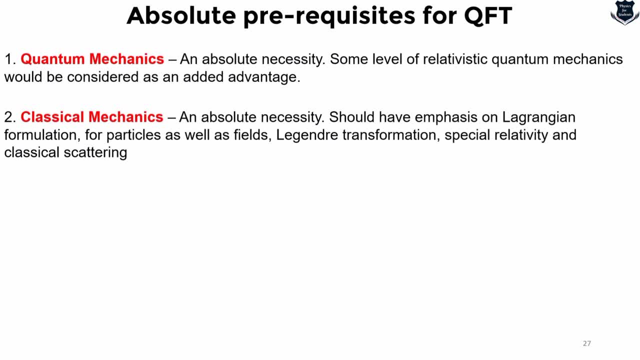 Next comes classical mechanics. Obviously You should emphasize on Lagrangian formulation, Legend of transformation, Special relativity and classical scattering Like baba scattering And things like that. You need to have an understanding of electromagnetism. It should cover Maxwell's equation. 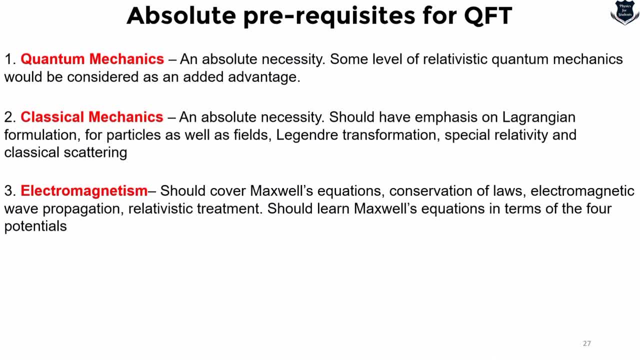 Conservation of laws. You know Maxwell's equations in the four Velocity or four potentials and so on. Relativity, Although not necessarily. I would request to have an idea About what is a covariant, contravariant. A little bit about metric tensor. 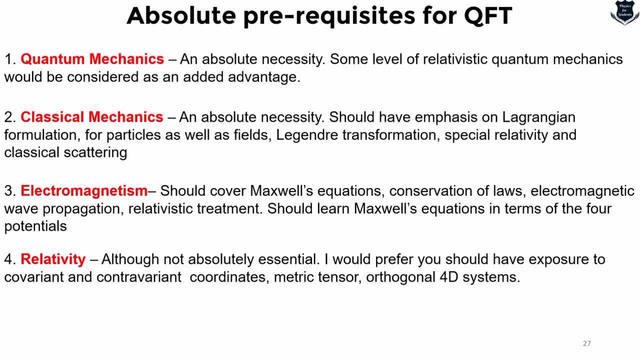 And all those orthogonal Four dimension systems. So these would be, I would say, An absolute prerequisite. Without that, It is impossible to go ahead With quantum field theory. Now, having said this, You might think that, okay, Let me go ahead and select a book. 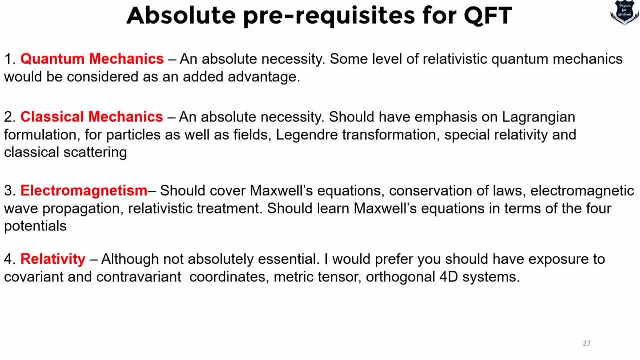 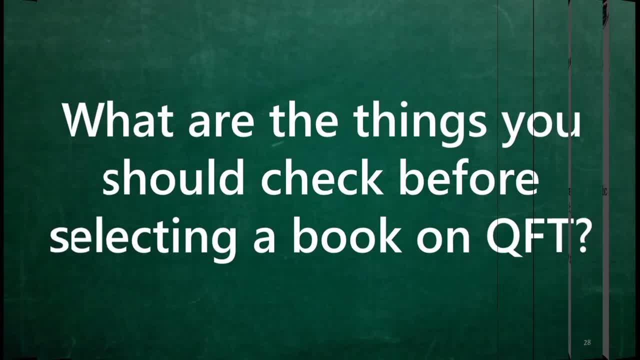 One single book Which will teach you quantum field theory. When you are going ahead and selecting a book on quantum field theory, What are the things you should check? What are the things you should keep in mind That this book should have Coming up into the next part of the video? 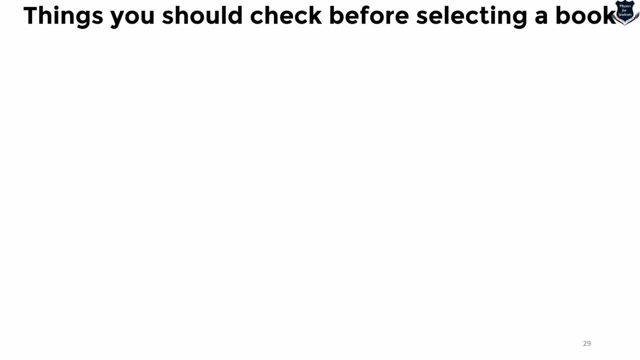 What are the things you should check Before you select any book in quantum field theory? Now, the first thing Is avoid brevity. Now, what I am trying to tell is that It comes as a horror for most of the students. Very brief. 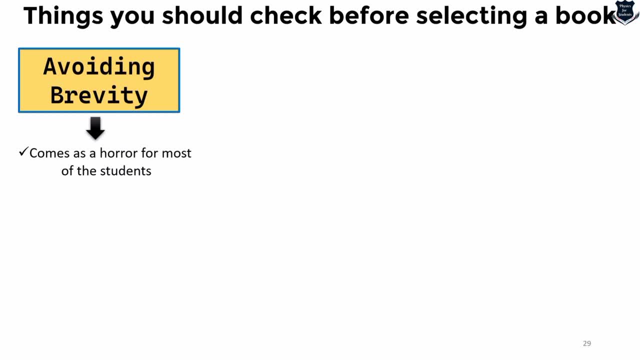 And a lot of brevitys are being used, Lot of signs, Lot of symbols which are being used Without having any explanation. It should be avoided. in some areas of physics, It should be more of elaborative, Very clear. That is why I wrote the last one. 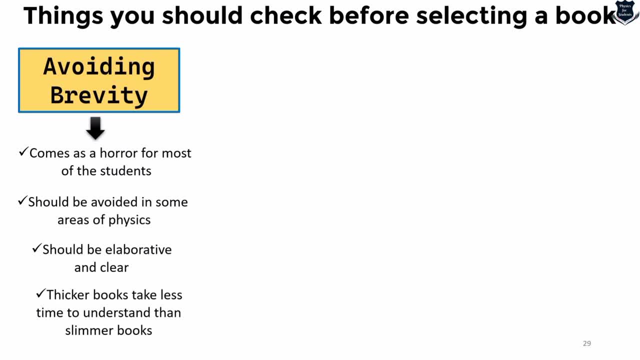 Thicker books are much less Takes less time to understand Than slimmer books, Much more elaborative, Literary and easy understanding. Slimmer books takes a lot of You know, Symbols, etc. into account. So look into a book which is avoid brevity. 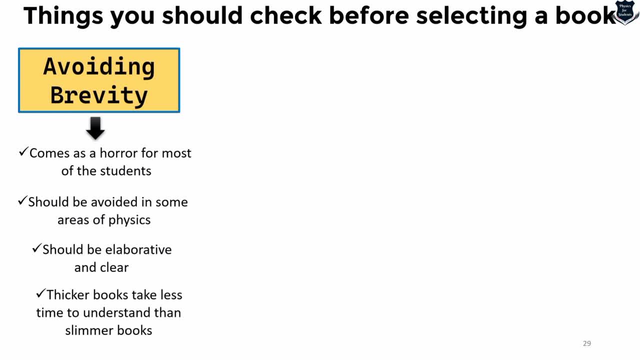 It does not have too much of Symbols and notations, But it expands and clears up the concept. Second is that The book should have a holistic approach. That means it should contain certain Non-mathematical overviews. There should be a big picture. 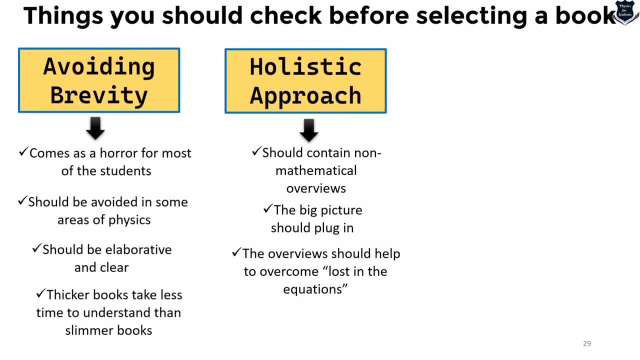 And the overviews should be To overcome lost in the equations. I mean to say, at the end of each chapter Or by the beginning of each chapter, The book should have certain overviews. That means what is More or less told into this chapter. 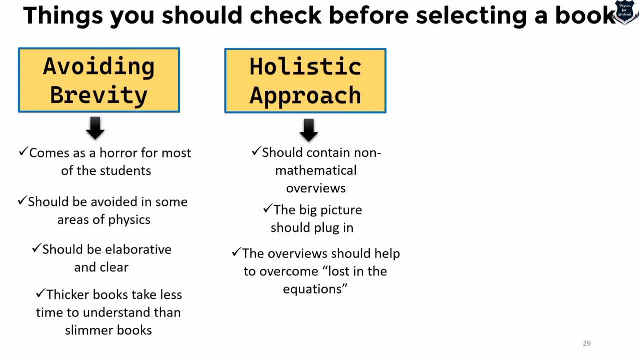 What is the summary? In a very simple language, Not using much equations, So that is why I use the word Lost into the equations, And there should be a check At each point of the book. The next thing would be Schematic diagram summaries. 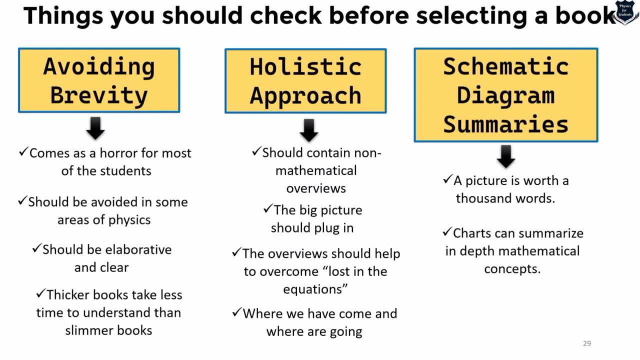 As we always know That a book picture is worth in thousand words And there should be charts So that we can summarize In depth mathematical concept And comparison, just like I told you, Between QN and QFT, A kind of a chart. 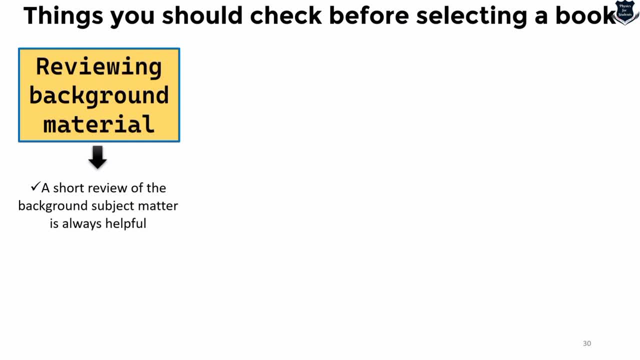 Which gives a better kind of a learning experience. The reviewing of background material: Yes, it is required. There should be a short review Before you learn this, So that you can understand What is the problem. field theory, A revision and revision. 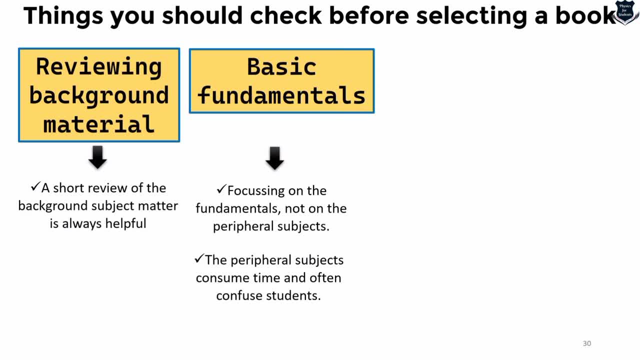 Of the fundamentals are required. The peripheral subjects Sometimes are elaborated so much That it consumes time, Students get confused And the main objective is not being served. There should be certain exercise Where there is a proper return on investment. That is not too much of exercise. 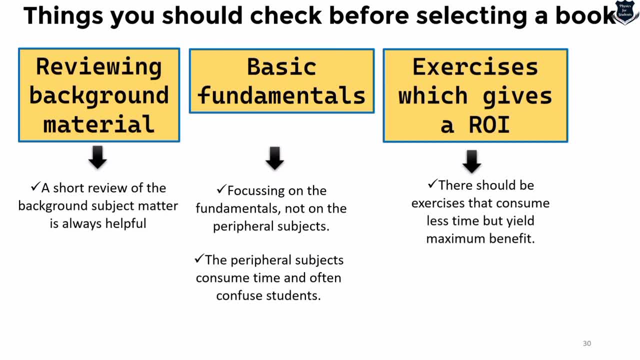 But certain exercise Which yields the maximum benefit. So, before you go ahead And read the book, If these things should be there, Then a book is fine and good enough In order to go ahead And for you to read Now. first thing is that 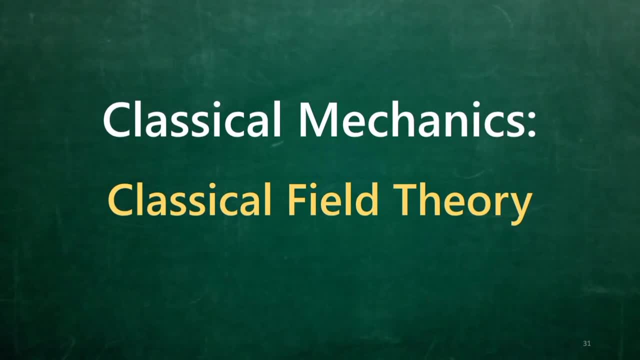 What we are doing is that We are now going to understand classical, I would say the quantum field theory, Taking into account What is called classical mechanics, And we should first understand a little bit, And we should also know what is the book. 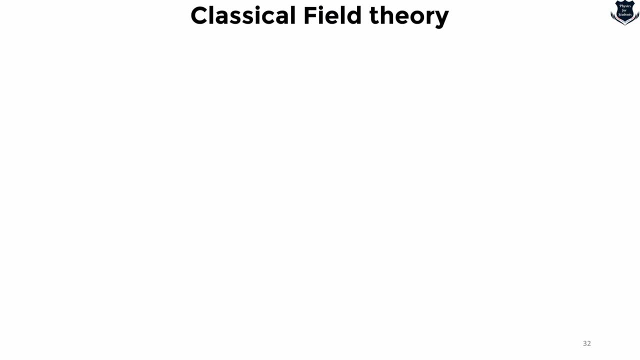 That we should read in classical field theory. We are supposed to go Into quantum field theory. Now you see, the thing is that In general, we are, Our brain is wired to treat things as particles. So if there are particles, There is a position. 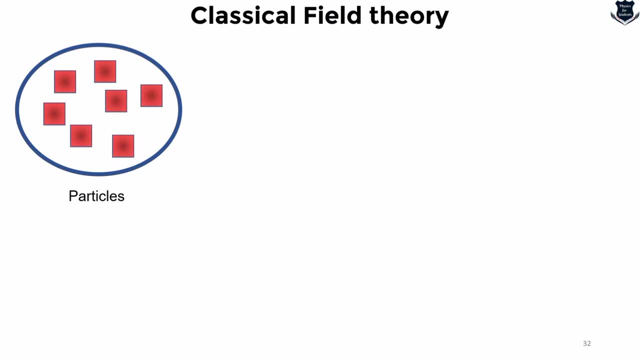 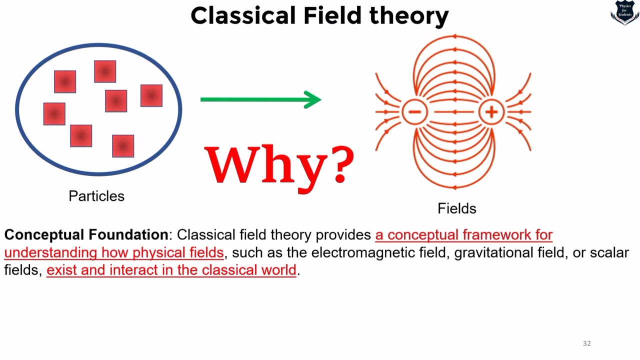 There is a Cartesian coordinate, There is a momentum, There is an angular momentum, And we are all quite comfortable in that. But you see, now Things are getting, I would say, Generalized into what is called a field, So conceptual, Going into fields. 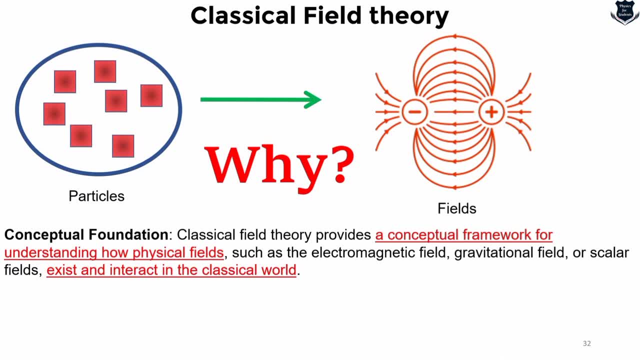 So classical field theory First we need to learn, Because it will provide a conceptual framework Of understanding how physical fields, For example electromagnetic gravitation and others, They exist and interact in the classical world. Because if you don't understand The classical field theory, 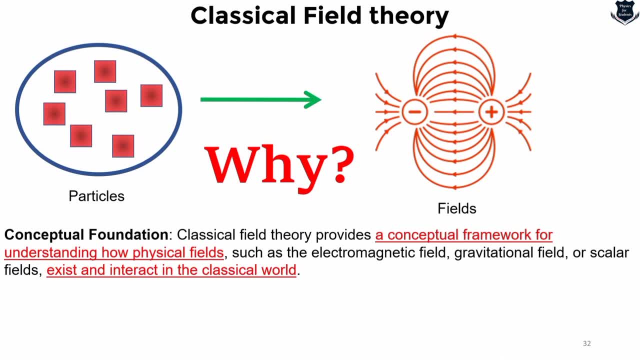 Then going into fields of quantum field theory Where there are lot of infinities, Lot of degrees of freedom, You will get confused. The second is that classical field theory Actually teaches you The mathematical tools, And these mathematical tools Will be elaborated in quantum field theory. 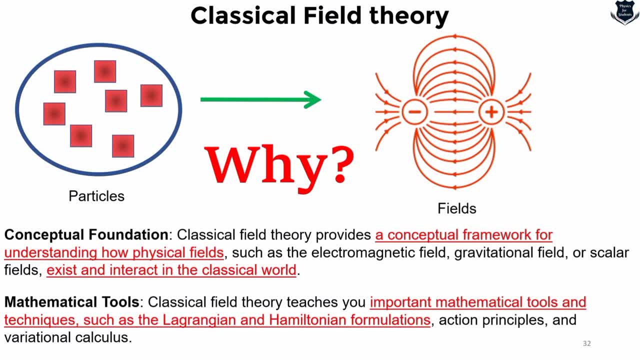 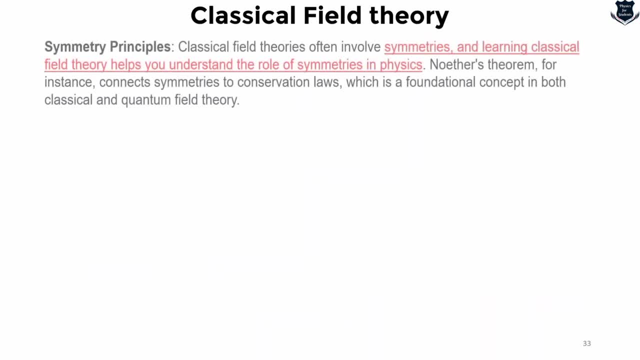 Such as Lagrangian, Such as Hamiltonian, Such as action principles And variational calculus. So a very good you know Understanding of classical field theory Is a must before we go into quantum field theory. Also, there are certain areas. 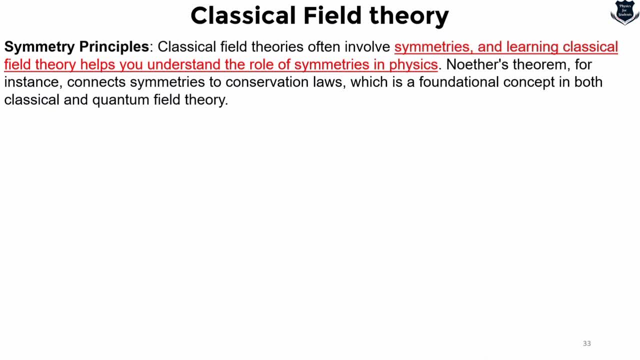 Which is called symmetry principles, For example Noether's theorem And other areas, which is very foundational. We will also deal with symmetries In quantum field theory, But understanding of classical field theory And classical symmetries are important. And quantization. 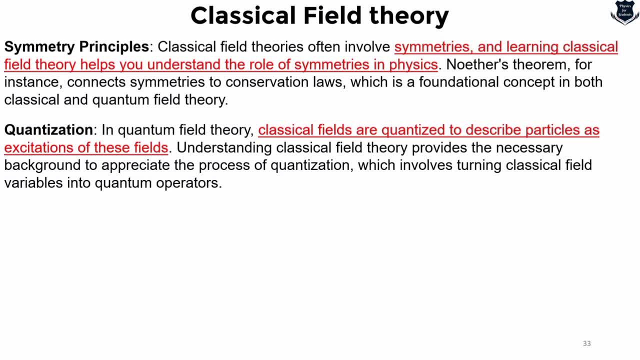 Yes, very important, Because classical fields are quantized To describe particles as excitation of these fields. So in order to understand The further quantum field theory, It is necessary to appreciate The process of quantization Which involves classical field variables. 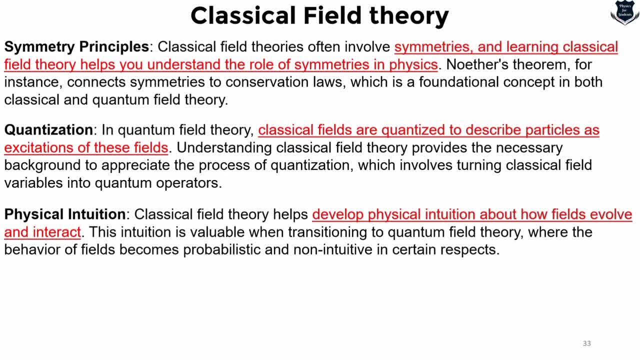 Which later turns into quantum operators. Lastly, We have a physical intuition. That means you close down your eyes And you visualize how fields evolve And interact over time. This intuition becomes very important Because when you transition from classical field theory To quantum field theory, 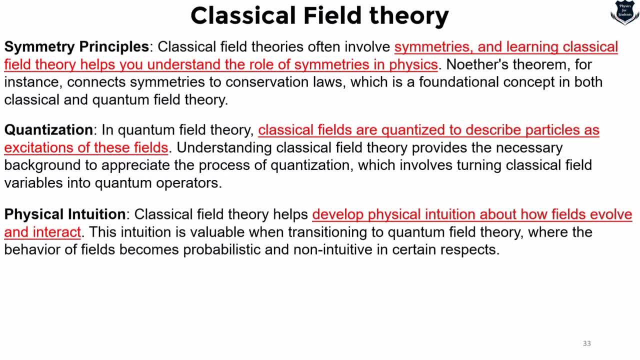 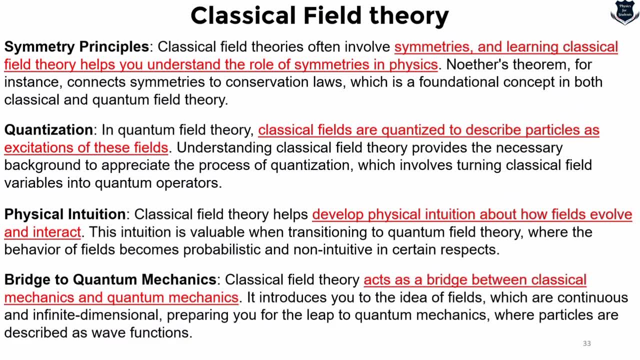 The behavior of fields become probabilistic And non-intuitive In certain aspects is required. So, finally, what we can tell is that It is also a bridge to quantum mechanics, Because classical field theory Is a bridge between Classical and quantum world. 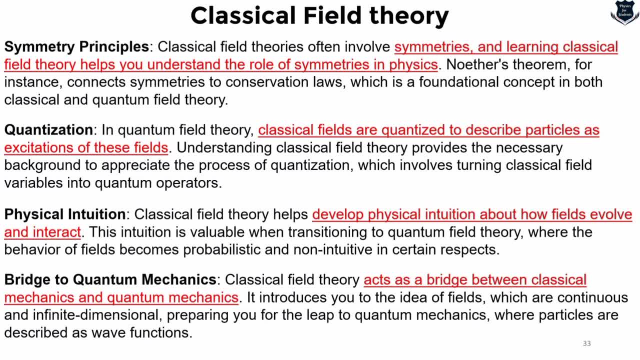 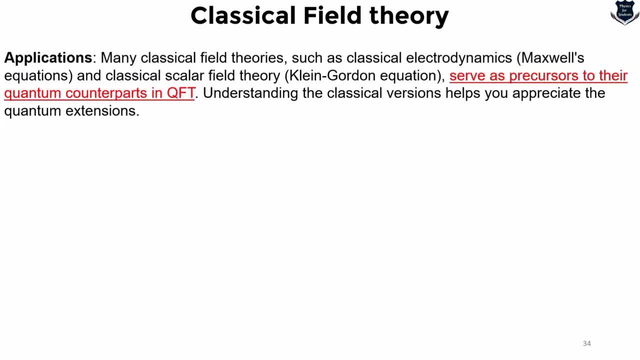 It gives you the ideas of fields Which will later become continuous And infinite dimensional And help you to prepare To leap into the field of quantum mechanics. Also the applications Many classical field theories Such as Klein-Gordon And Maxwell's relativistic equation. 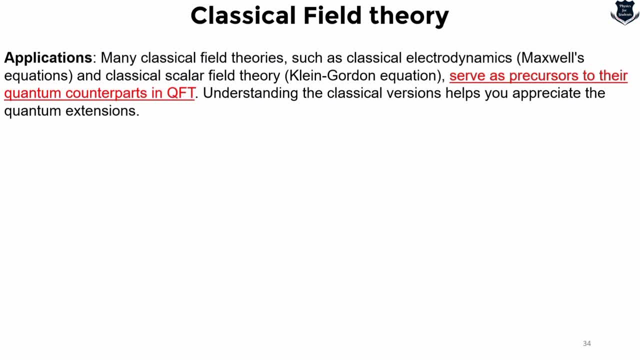 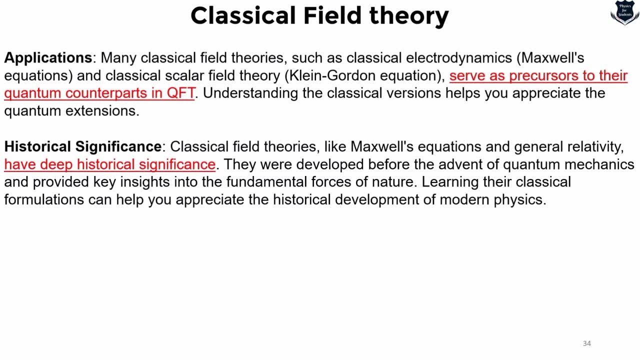 Serves as a precursor. That means you are getting ready yourself Into the quantum counterparts Of quantum field theory And obviously, as I have always told, You learn what is the historical development And how actually classical field theory Generalized And become much more advanced. 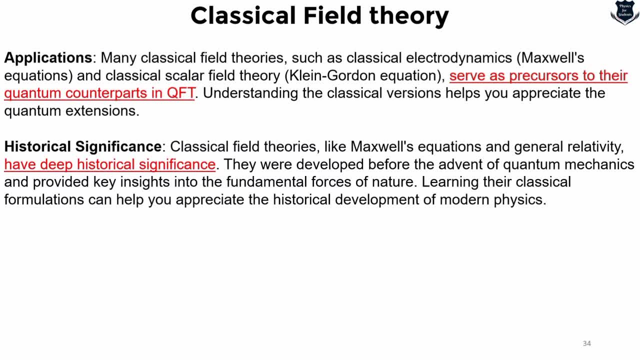 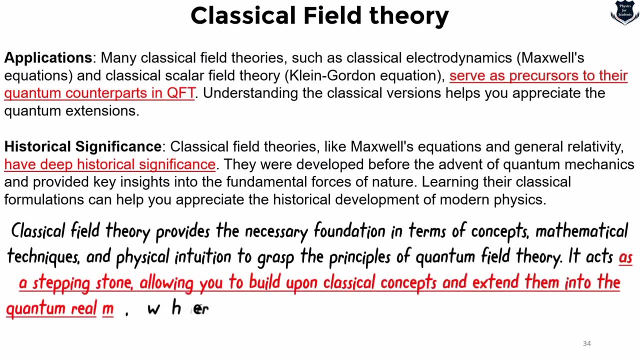 In quantum mechanics And later into quantum field theory. So, taking everything together, What we can tell is that Classical field theory actually provides The basic foundation. you need The mathematical techniques And the physical intuition In order to grasp quantum field theory. 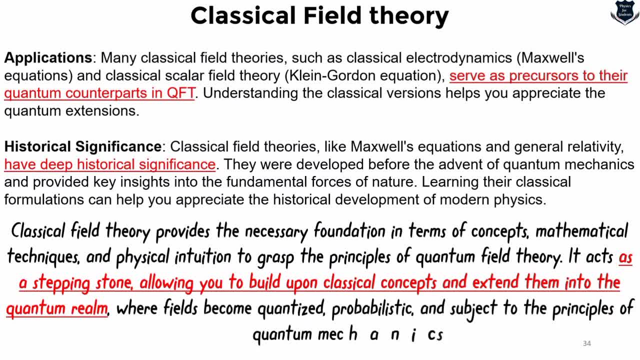 It also acts as a stepping stone Which allows you to build upon The classical concepts And extend them to the quantum realm. So this is the first thing. I will come to the book part In this video quickly. But this is the reason. 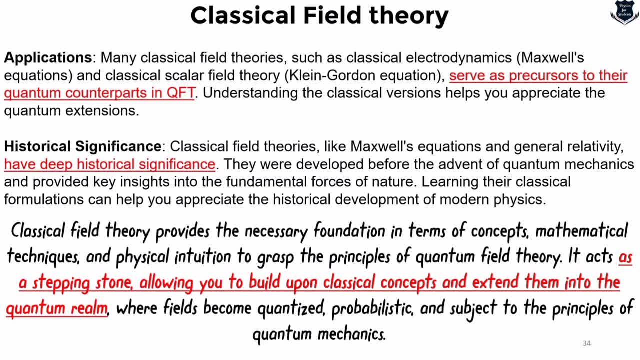 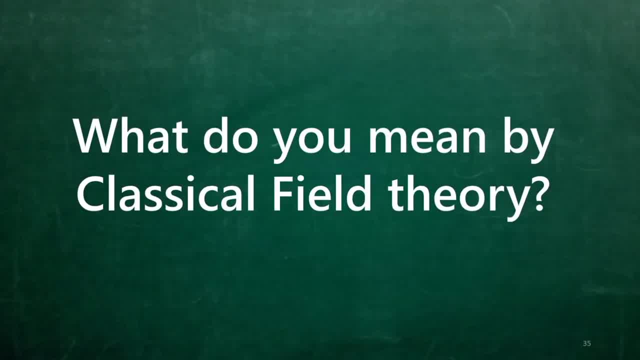 That you should not ignore classical field theory. Learn, understand, Because that is the stepping stone On which classical field theory will be built. The question is that: What do I mean by classical field theory? When I am telling it, What do I actually mean? 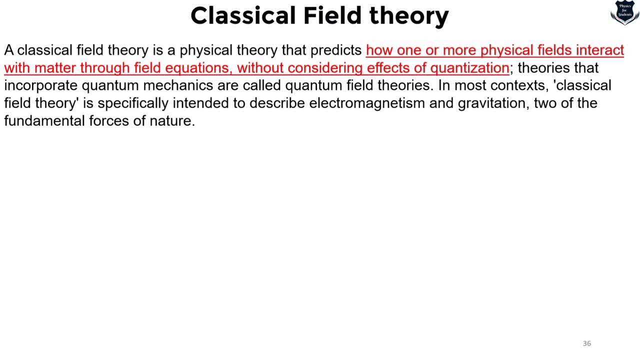 Coming up into the next part of the video, I am going to tell you How the quantum fields interact with matter, But without quantization, Obviously. when it is quantized It would not be a classical, It would be quantum. So classical field theory is specially intended. 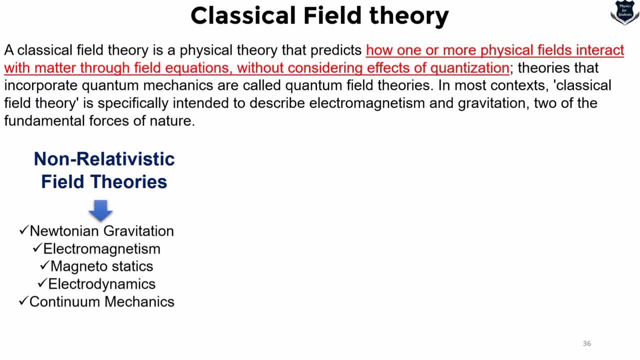 To describe electromagnetism and gravitation, Two basic fundamental forces. So in the non relativistic arena There is Newtonian gravitation, Electromagnetism, Magnetostatistics, etc. In the relativistic field theory We have got electromagnetism. 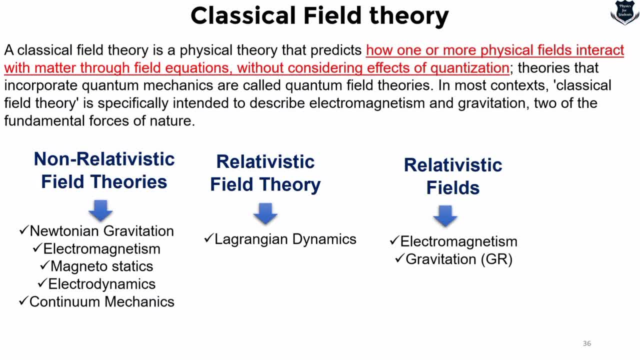 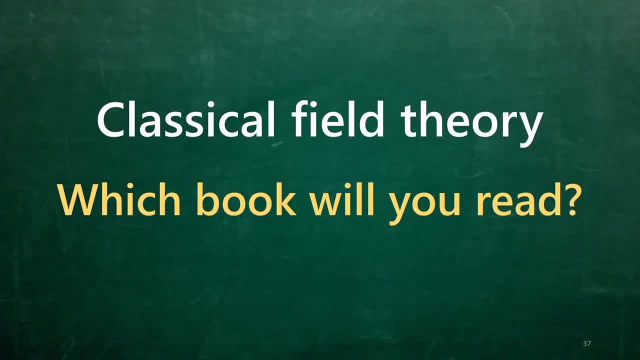 And gravitation. So now it is the time That we should go into selecting What is the right book Which will help you to learn classical field theory. Which book will you read? Coming up into this part of our video Now, I would straight away go. 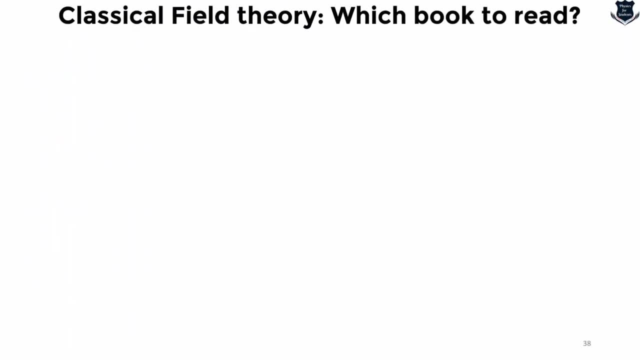 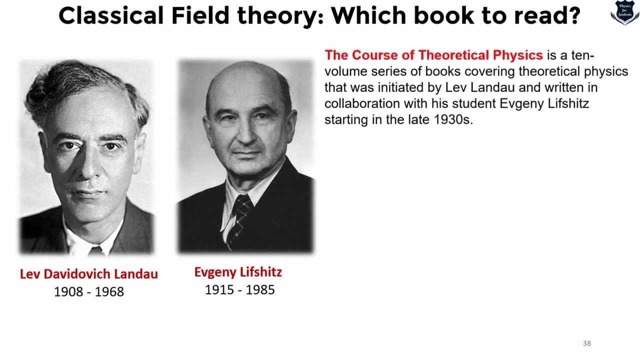 Into classical field theory, The very old, The very classic, The very famous book of Landau and Levjits. Now, this Landau and Levjits Actually created a phenomenal series Which is called A course of theoretical physics. Now it is said that Landau actually composed. 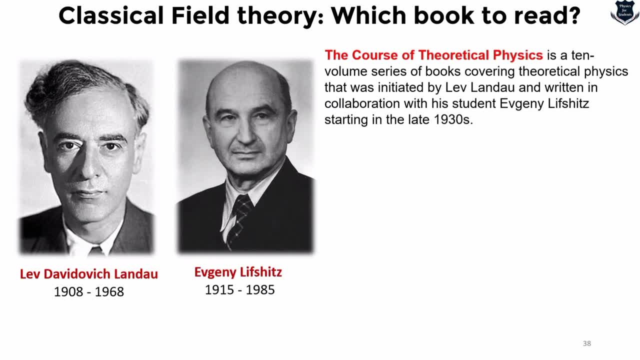 Much of the series Staying in this NKVD prison During 1938 and 39. And almost all the actual writing Of the early volumes was done by Levjits, Giving rise to this famous witticism: Not a word of Landau. 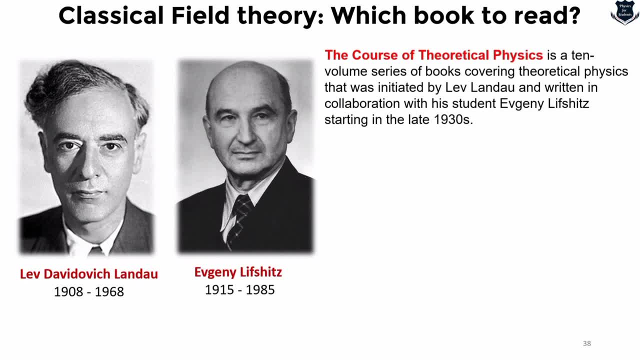 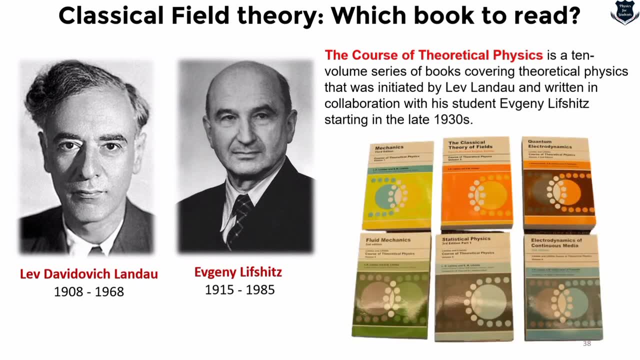 Not a thought of Levjits. So the first eight volumes Are actually finished in the 1980s. This is kind of a. You know It is written by Russian And you know who translated it in English. It was none other than. 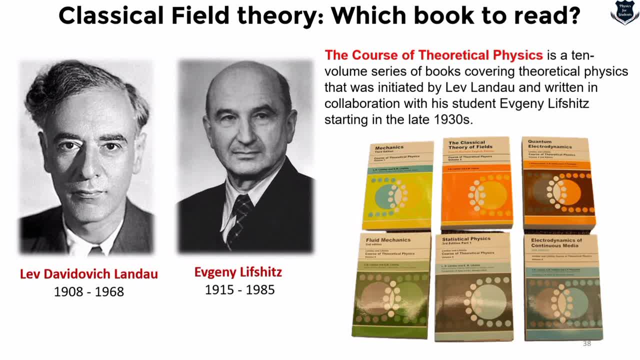 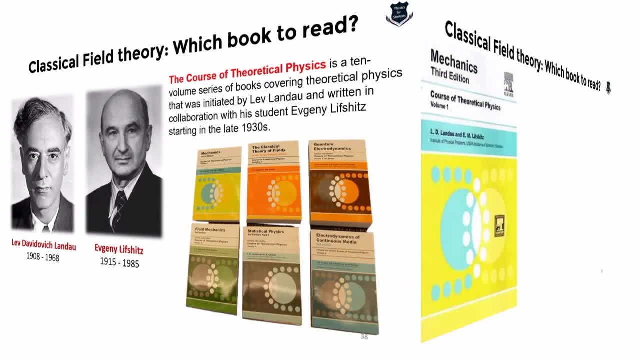 John Stewart Bell, Who is known famous for his Bell's theorem. So this is A kind of a book Which I would request you can go. And what is the name of the book? Let us look into it. The first volume actually is the classical mechanics part. 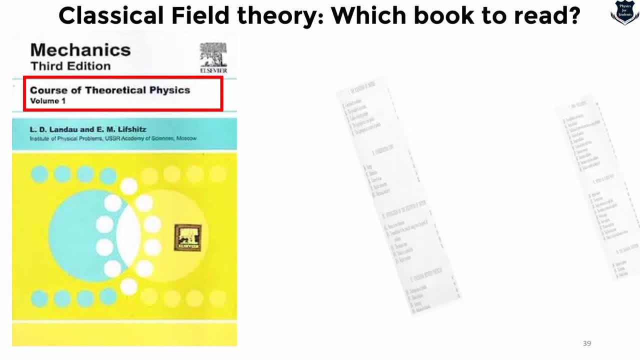 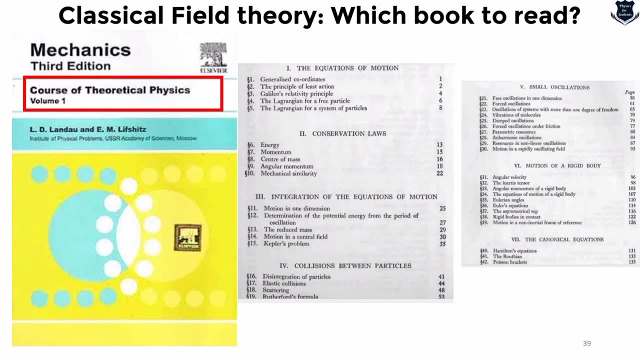 You can go into it. I mean to say there is no harm in going into it, But it actually contains these type of You know topics: Conservation of laws, Collision between particles, Oscillations And the canonical equations. So this is just, I mean to say, the first part. 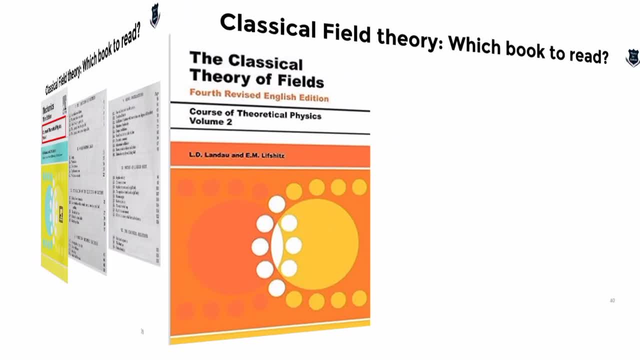 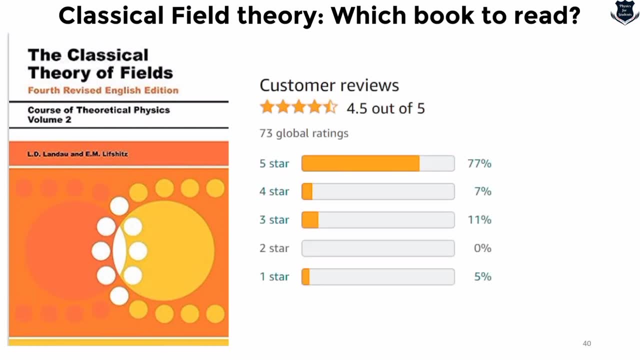 Of Landau Levjits And it actually comprises the classical. We are more concerned with this one Course of theoretical physics, Volume 2. Which it deals with classical theory of fields. Now, overall, if you see the Amazon rating, It goes 77%, 5 star. 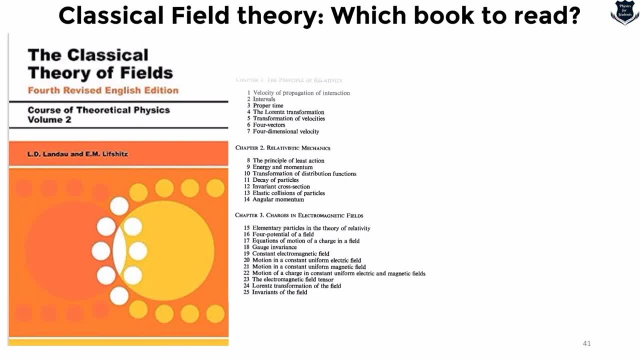 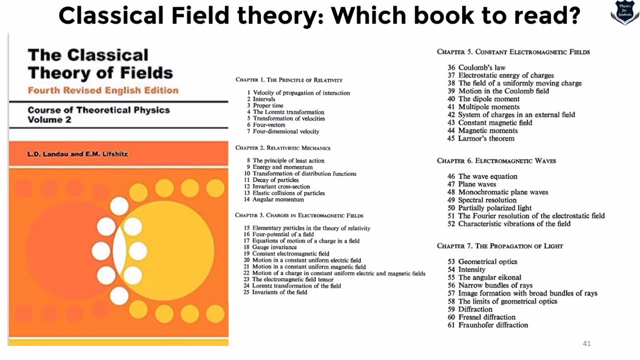 And rest of them. So what is the content? It is something like this: The principle of relativity, Relativistic mechanics, Charges in electromagnetic fields. It covers. it is very dense, I would say around 60 pages or so, If I remember correctly. 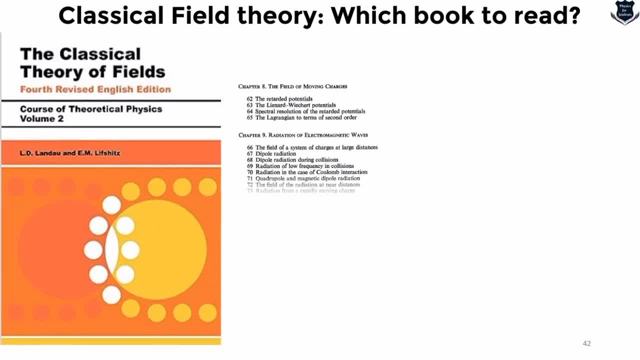 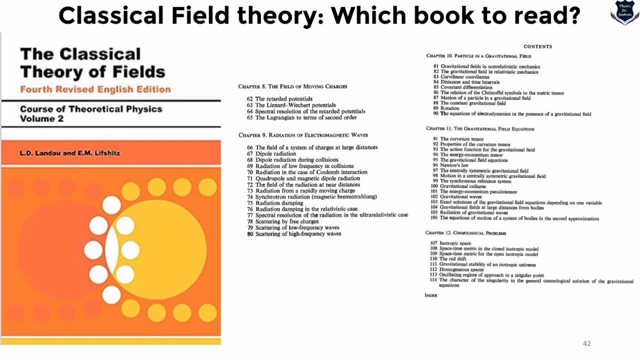 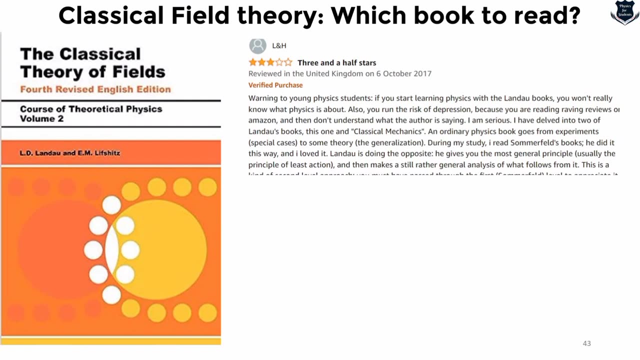 Constant electromagnetic fields, Electromagnetic waves, propagation of light. Further it contains the field of moving charges, Radiation of electromagnetic waves, And it goes into gravitational field, Gravitational field equation And some of the canonical problems. Now you see If I take the overall idea of this book. 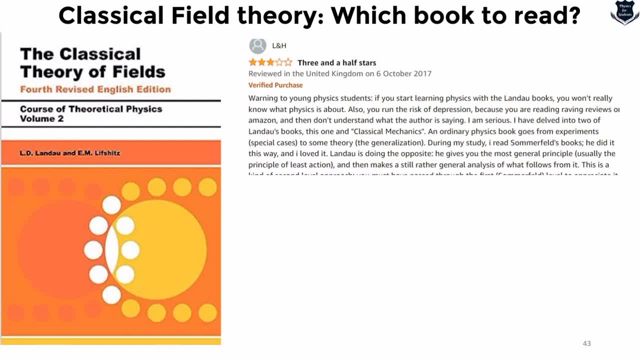 If I collect the best reviews, Then it says that It is a warning to young physicists. If you start learning This is this with Landau books- You won't really know what physics is about. And then it deals with, You know, into classical mechanics etc. 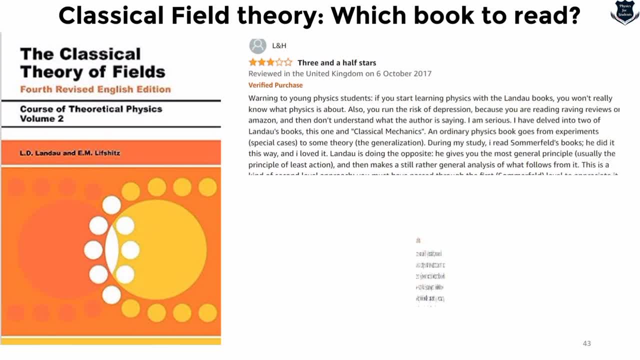 So this review tells more or less. It is not a kind of a suggested book, Due to some. The next Amazon review shows that Landau's approach to classical field theory, And I would recommend this title To those who are working in knowledge. 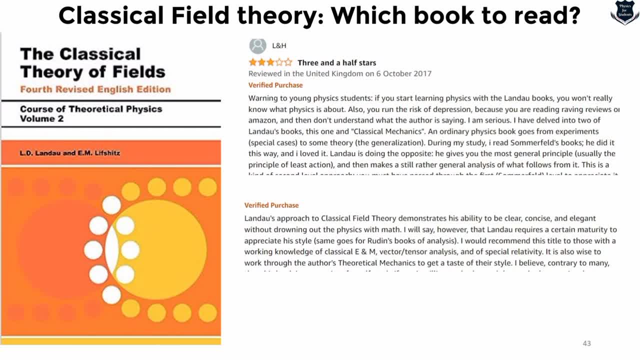 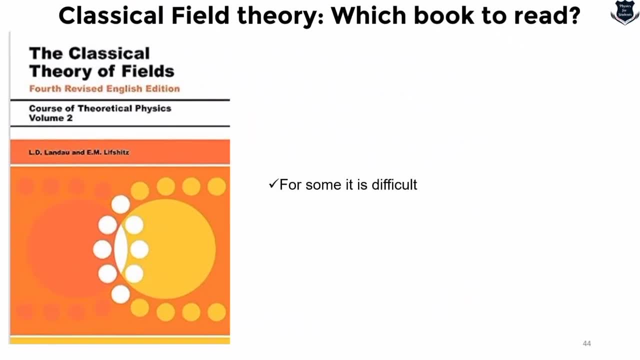 In classical electromagnetic vector and tensor analysis. So this also gives Not a very good review of this book. So after having read Through the Amazoncom and Amazon India, What I see is that For some it is a little bit difficult. It requires a good amount of mathematical knowledge. 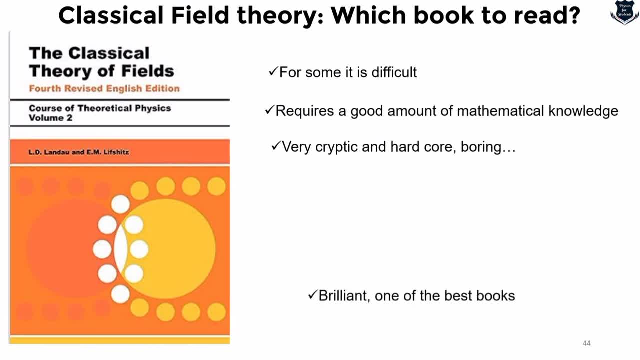 Some says that it is very cryptic, Hard core and boring. Some says it is brilliant And it is very clear and crisp and detailed. So you know, It is a kind of a mixed reaction. So obviously we cannot go through a book. 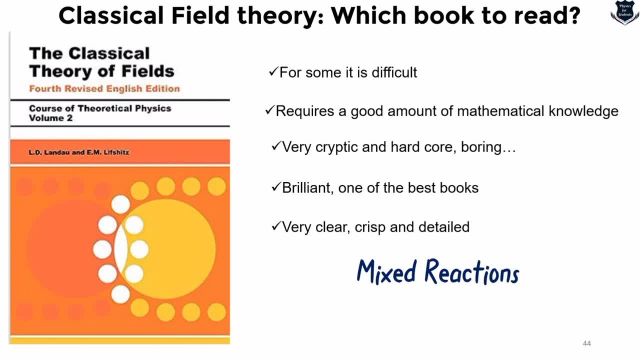 Which is called a mixed reaction. Some says it is difficult, Lot of equations, Some says it is brilliant. So question is that: Is there an alternative? Is there a book which will not go into any kind of a mixed reaction But just tell it is a wonderful, brilliant book? 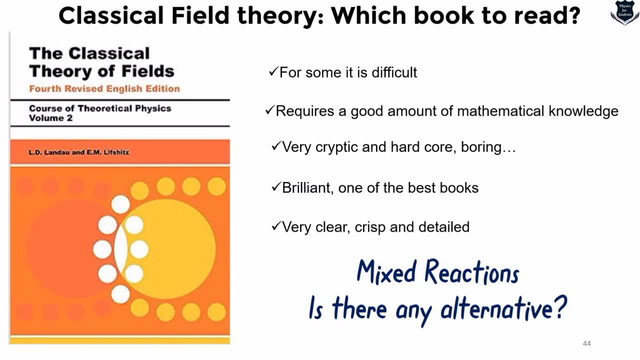 Yes, there is a book coming up in the next part of the video, But I would also like to tell Those who are mathematically inclined This is one of the best classic. This is worldwide celebrated. There is a collection of 10 theoretical physics books. 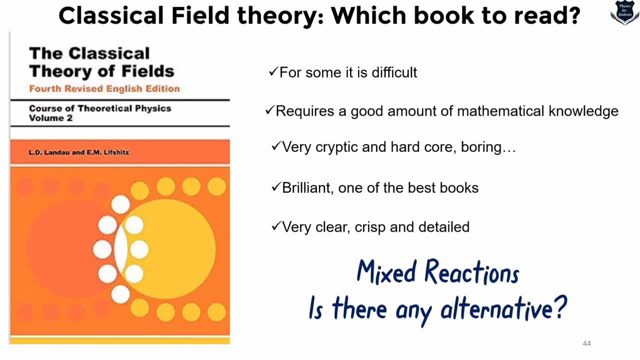 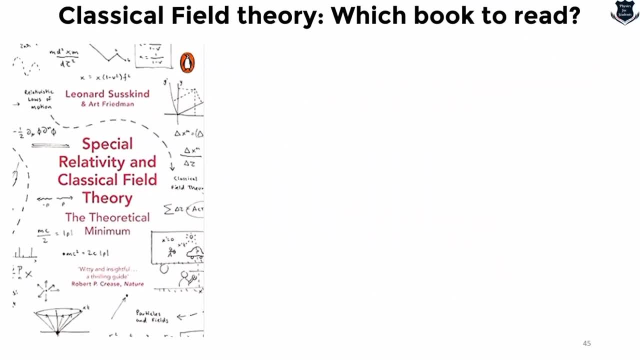 Starting from part 1 to part 10.. However, you can go into it. But yes, there is an alternative Which tells everything great, And this is none other than our dear professor Leonard Susskind. Special relativity and classical field theory. 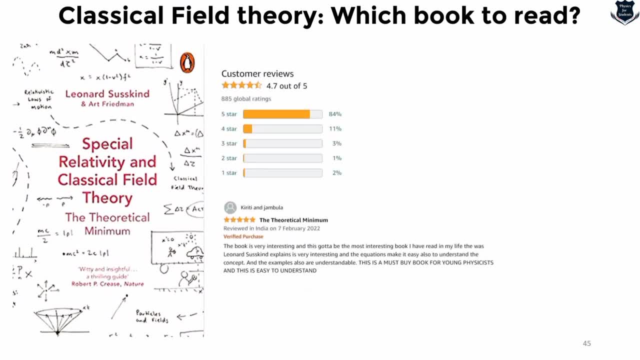 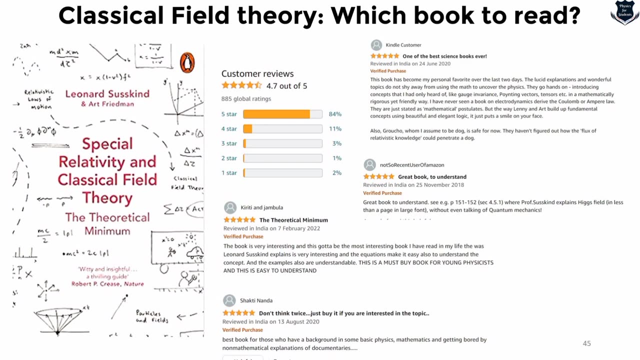 Check out those reviews. Everything Everybody says it is brilliant. The book is very interesting. The second text, The best book for those who have a background in some basic physics. This tells one of the best books, Science books ever. Great book to understand. 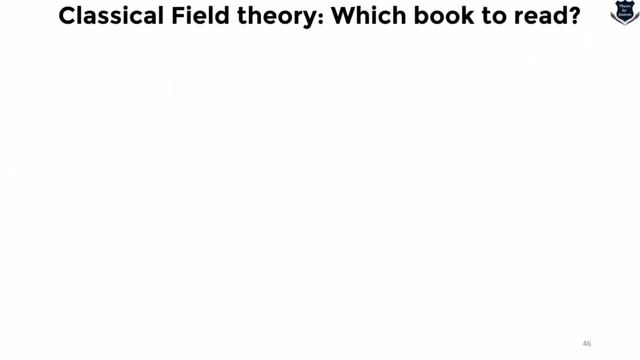 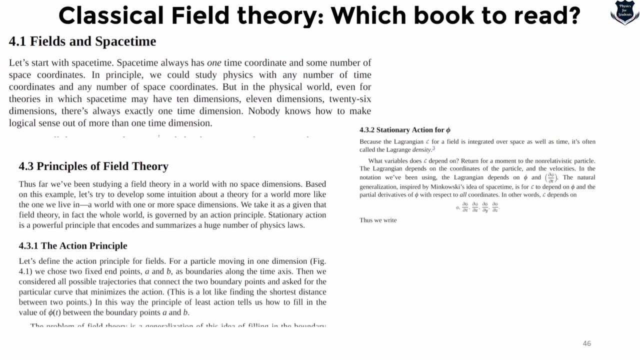 So obviously you can understand. This is very easy And it is appreciated by everyone. So you see that it starts with fields and space time. Then it goes into principles of field theory, The action principle, Stationary action, phi. That is the fourth part. 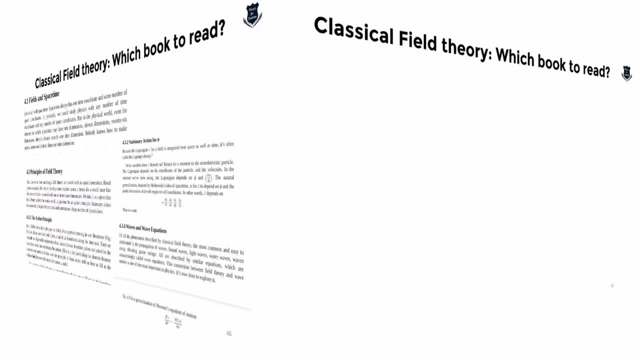 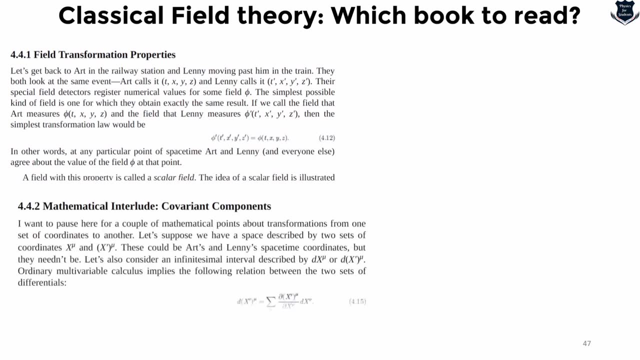 And it goes on. It contains waves and wave equations: Very simple, elegantly written, Clear and crisp, No problem in understanding. It has mathematical interlude of covariant components, As I told you, covariant and contravariant. In some aspect it is required. 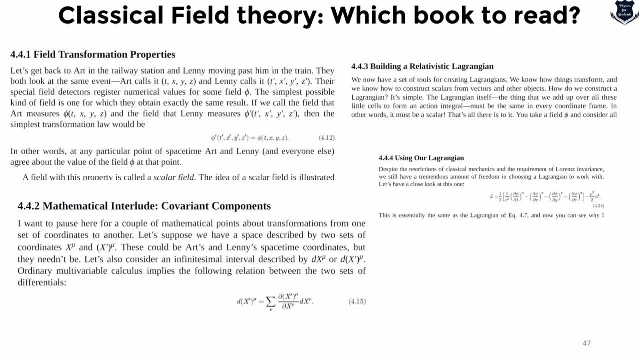 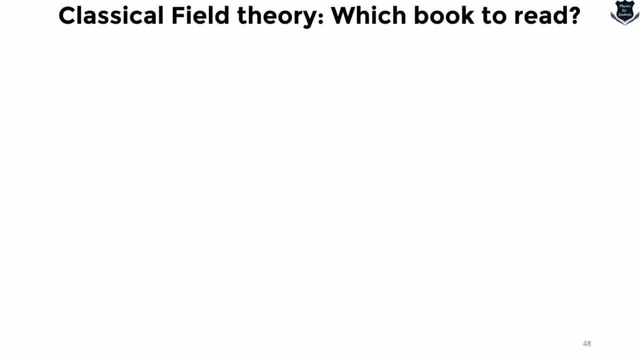 And it builds up the Lagrangian, Relativistic Lagrangian, Using our Lagrangian And the mystery field Which involves other areas of classical field theory. It uses nice diagrams Which are very clear to understand Field effects. 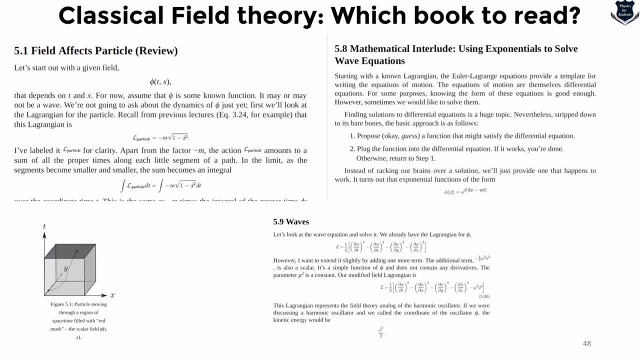 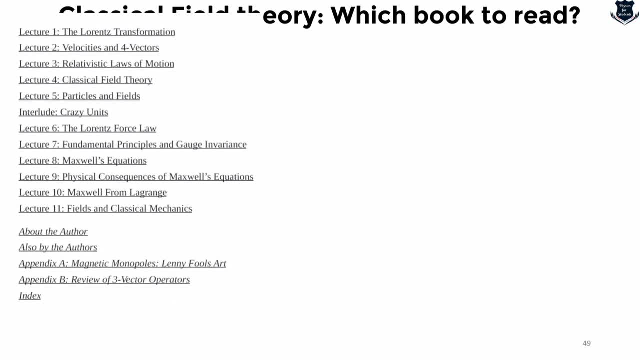 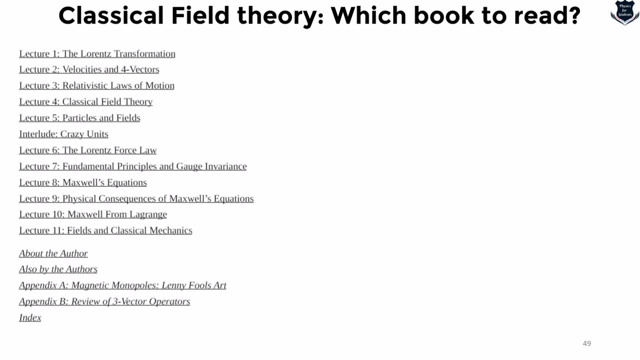 The review, Then the mathematical interlude Using exponential to solve waves and what not. So what I can say, This is basically the content of the book. It starts from Lorentz, transformation, Velocity, Four vectors, Classical field theory. It is comprising of 11 chapters. 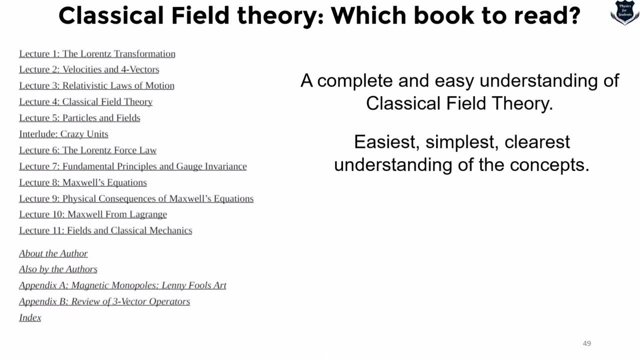 But very crisp, And I think this is one of the best book Which you can understand about classical field theory: Easiest, simplest, clearest Understanding of the concept. Whatever adjective I would use, That would fall less. So it is a very highly recommended. 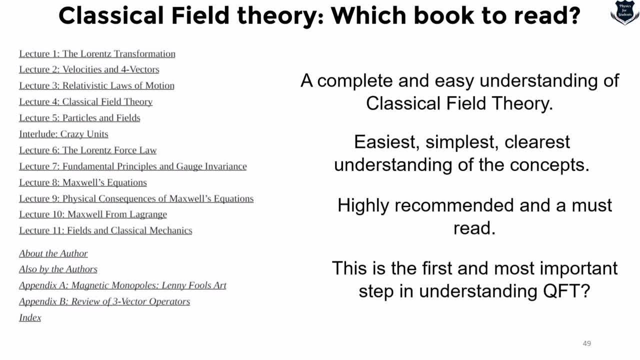 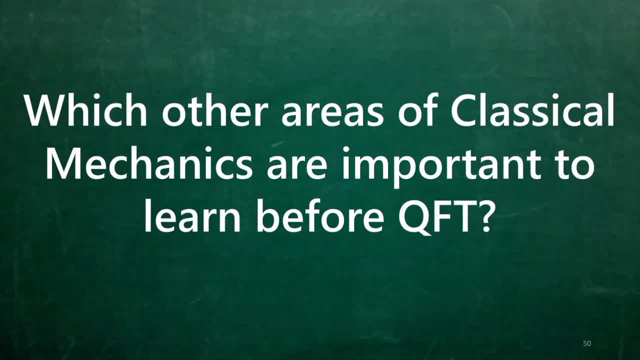 If you are interested in understanding quantum field theory, Without going ahead with this Basic part of classical field theory, We cannot go ahead with the second part Of the quantum field theory. Now you might have an You know kind of a question that